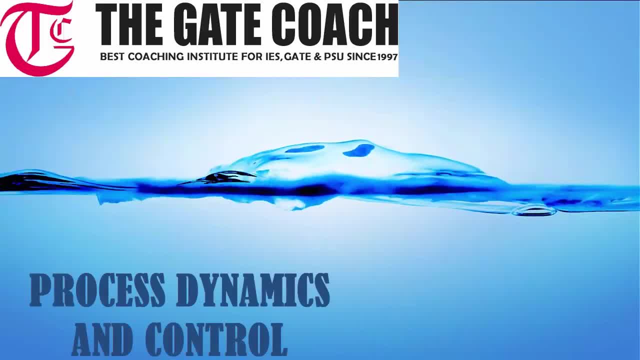 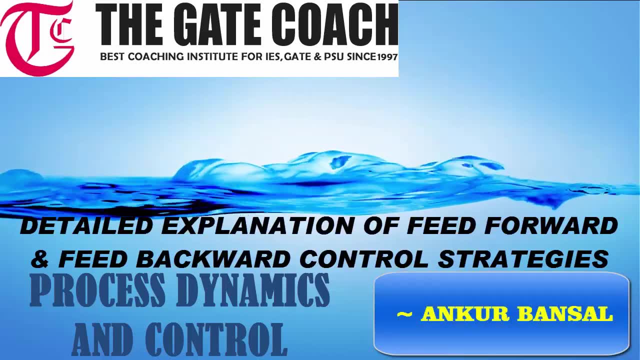 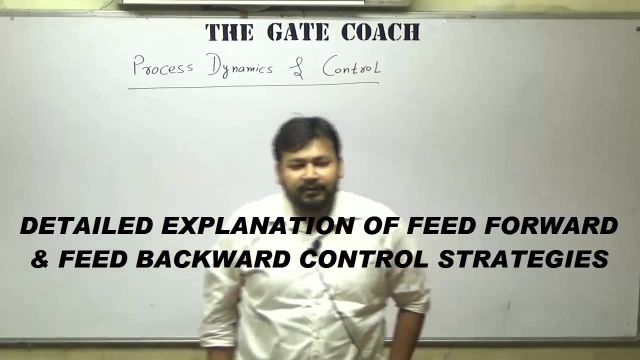 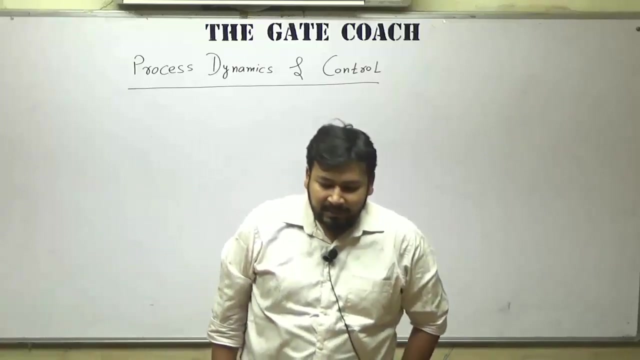 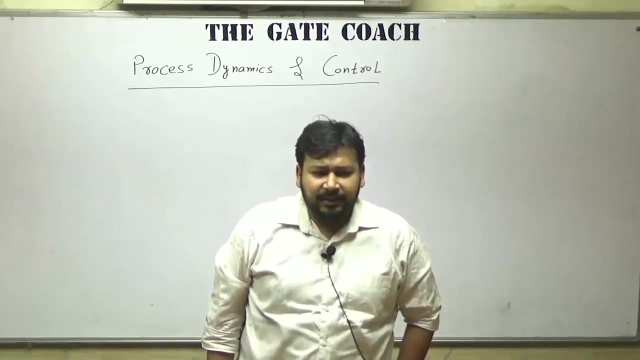 Good morning class. Today I am here to make a video on process dynamics and control, and in that there are many topics, many topics that are asked in the IITs for the MTech interviews and also for the GATE experience. the topics are very, very important. So one of the very 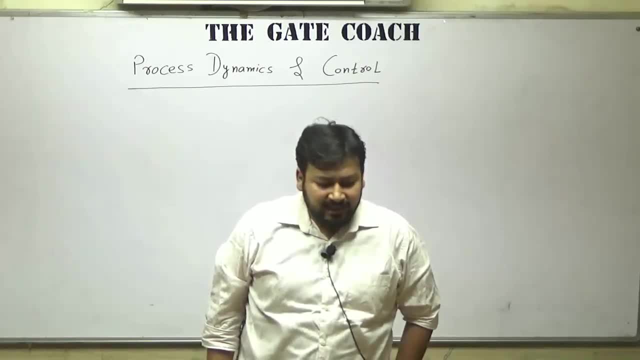 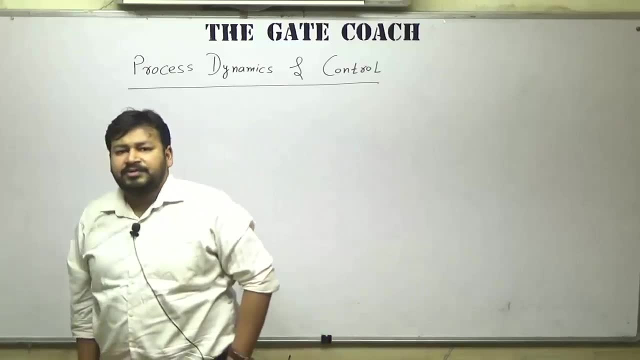 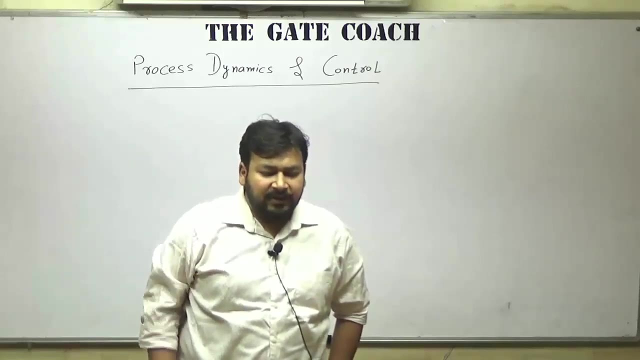 important topic is the designing- designing of the control system. So if I talk about the designing of the control system, there are many important steps. The first step we should need to take is the aim or the purpose. That means, what is the objective of our designing? 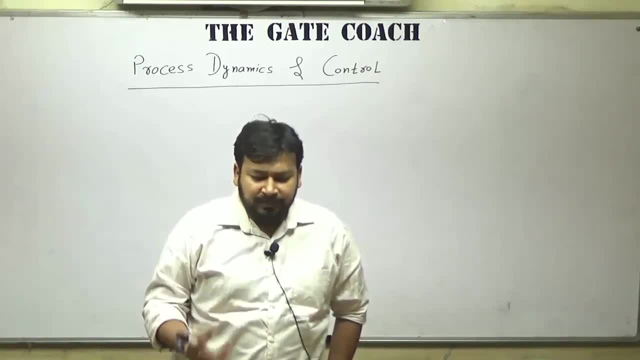 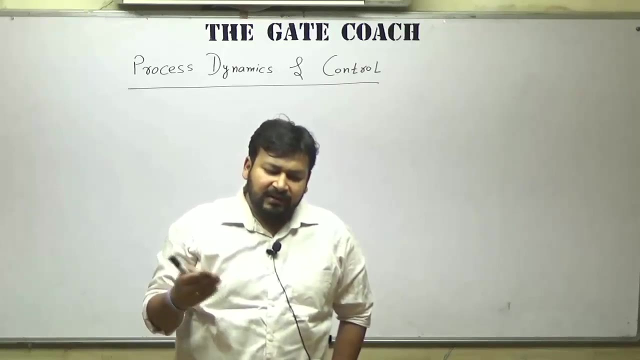 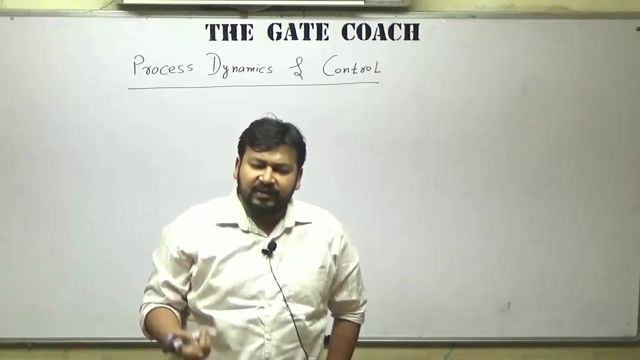 After deciding the objective of the main process, then we need to find out the measuring variable that to satisfy our aim, to achieve our aim, what should I measure so that I can fulfill my aim? So that is the second important decision. It comes in the designing part. The first thing is the deciding the objective variable. 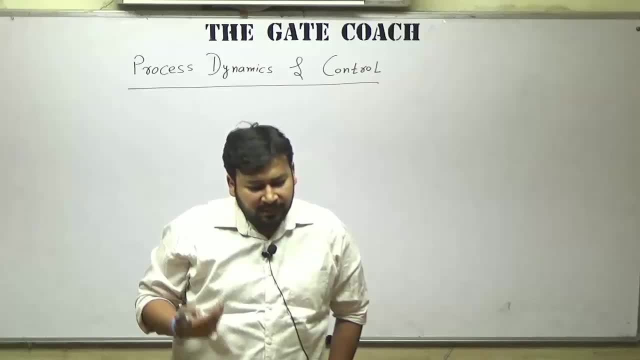 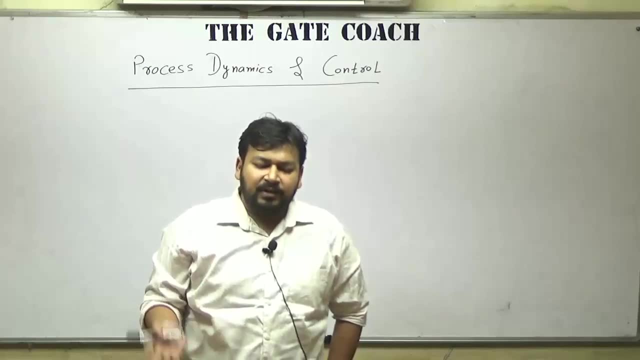 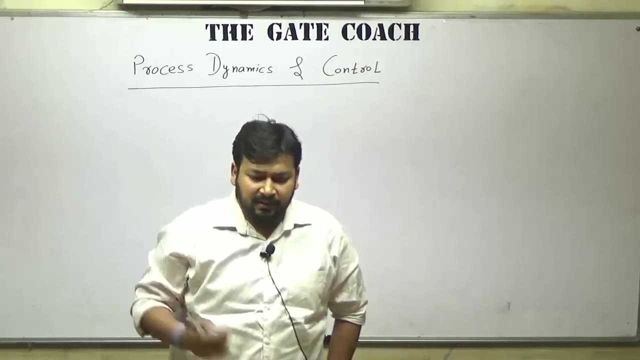 The second part is deciding the measured variable. Then the third important decision we take is the manipulative variable. That means what is that variable? by controlling which we can fulfill our aim or we can achieve our desired thing. So these are the three main decisions. 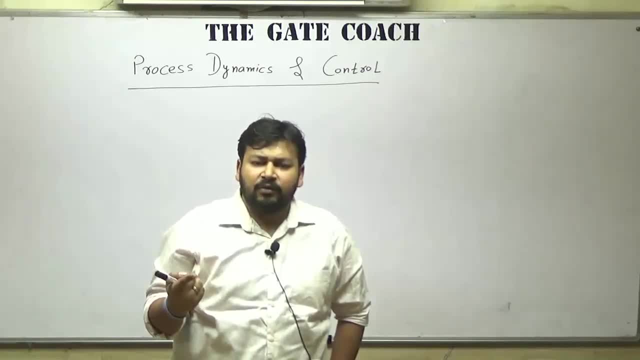 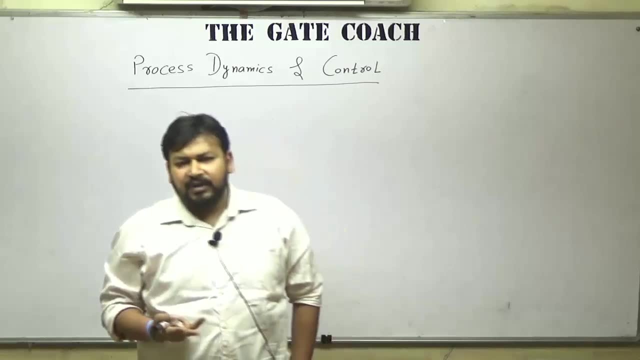 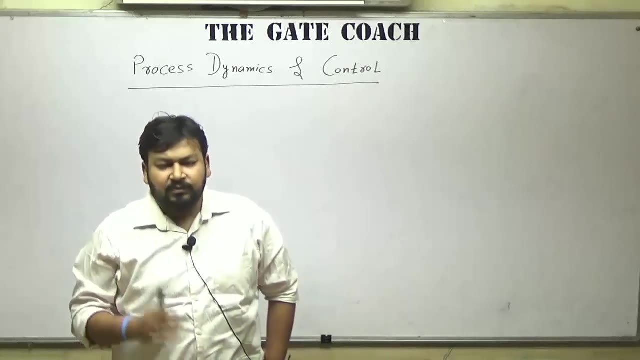 That is, the selection of the objective variable. You can say also the control of the aim, You can say also the controlled variable. Then second important decision is selection of the measured variable. And third important decision is selection of the manipulated variable. And after the selection of all these three, the fourth and the most important thing comes. 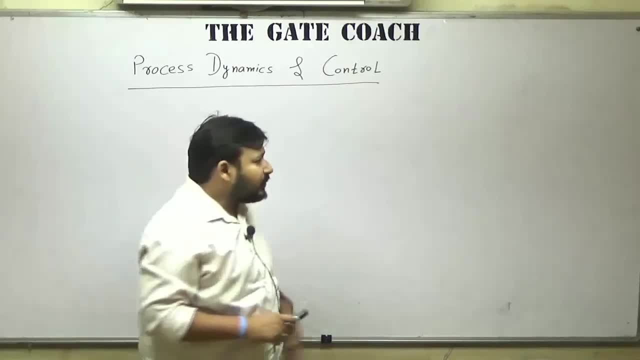 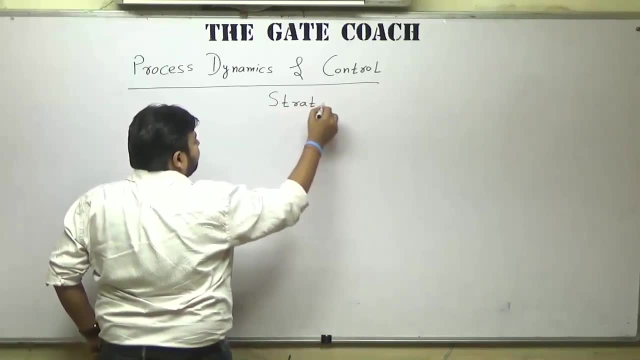 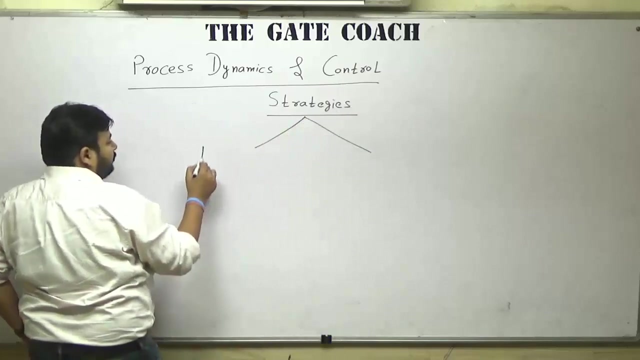 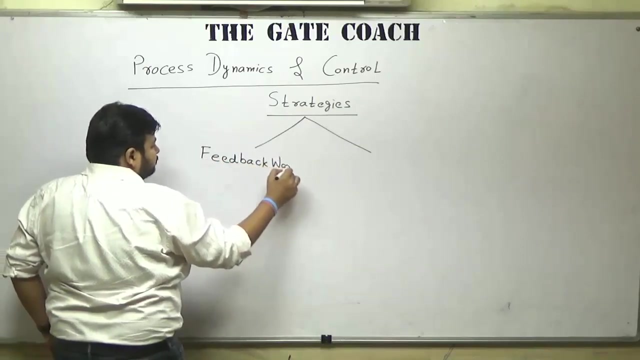 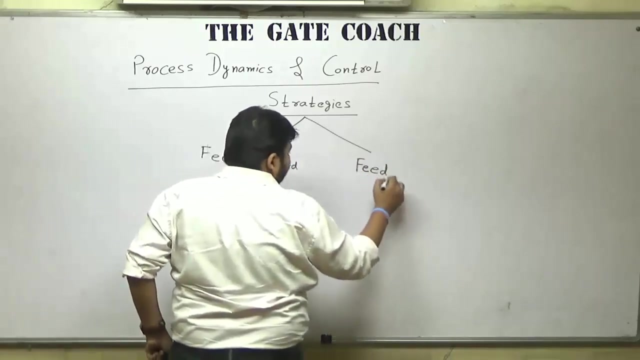 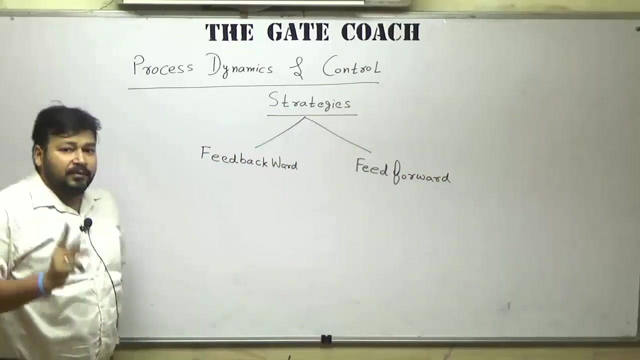 is the selection of the strategy. So here we are going to discuss about the strategies which, in the case of control, are of two types. First is known as feed backward, other is known as feed forward. So remember, when the strategy comes, it is the fourth point, The- 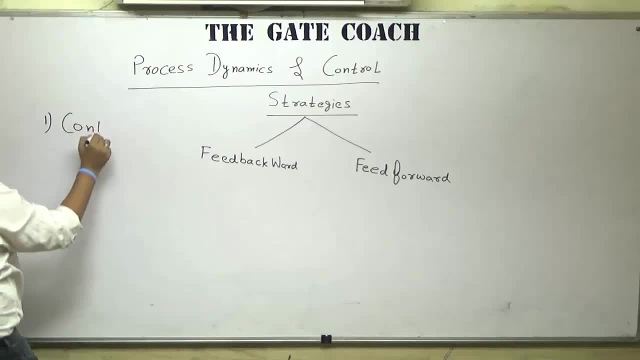 first point is controlled variable. The second point is controlled variable. you get the second level point mentioned here. controlled variable is a given by the. then what is important is the measured variable. The third one is the manipulated variable, And you also remember this. this we can consider by the one, by one. 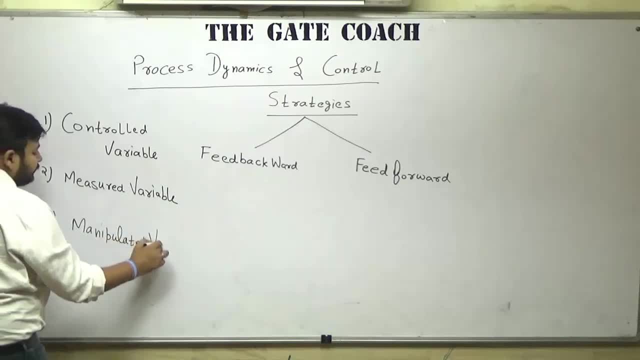 Okay, Let us consider financial. and, last but not the least, We cannot consider financial and, last but not the least, Next Wednesday, the mitral ftc time. When you add the real run out agents, when you add this one, the market that increases. 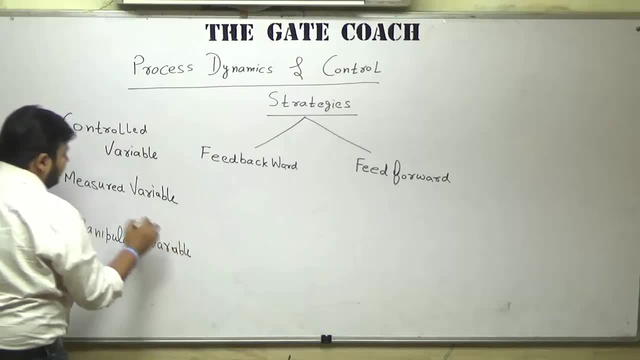 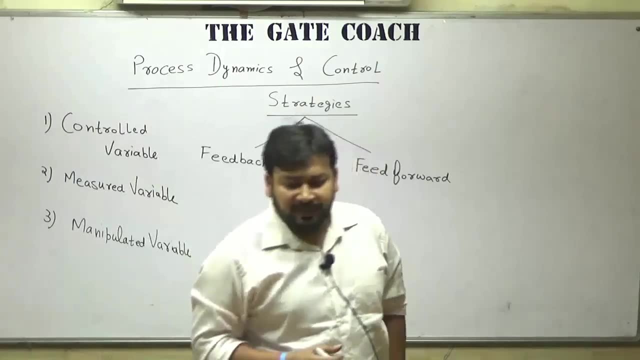 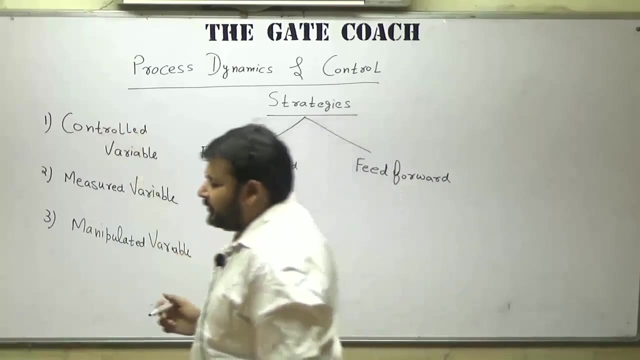 all over the market. So this is the third point. you want to know about all these three: what is controlled, what is measured, what is manipulated. if you want to know more about them, you can comment in the comment section. i will make a separate video by for explaining all these three, but these are the key decisions. these are. you can. 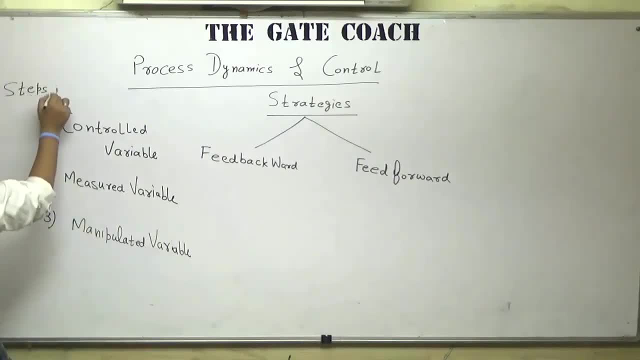 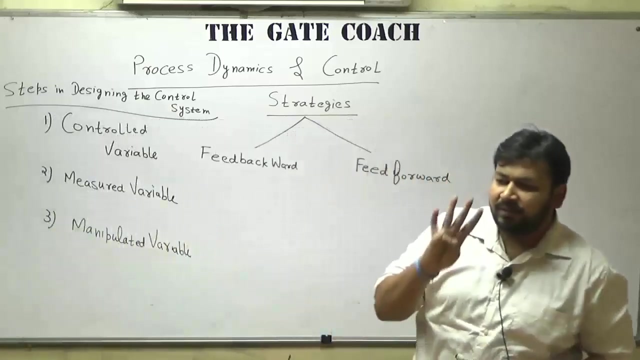 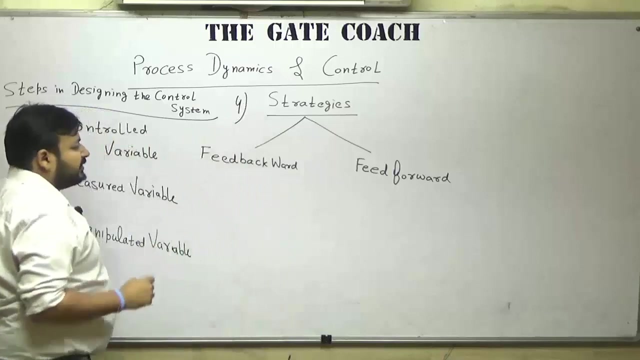 say the steps: steps in designing, steps in designing the. so first three steps are these steps. if you want to know more, i will make a separate video on them. but the fourth important step, that is, very, very important step, is the selection of strategy: what strategy we should take, what strategy we should apply so that our control 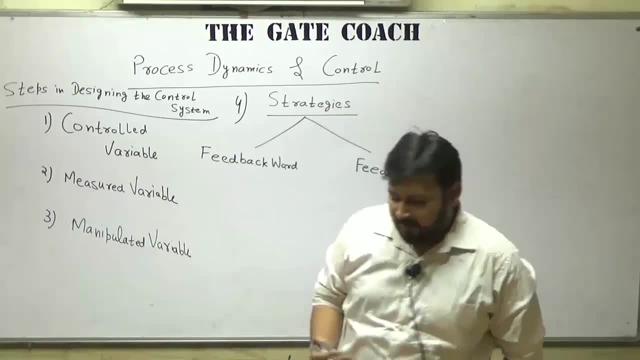 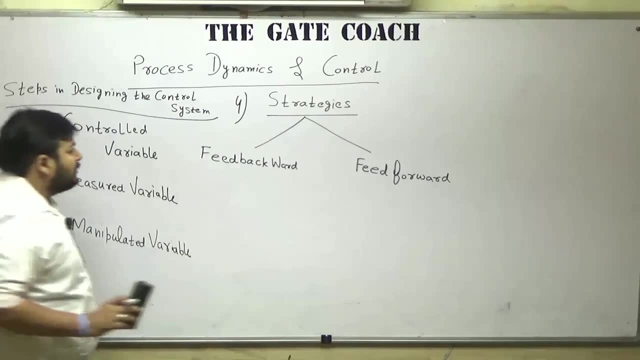 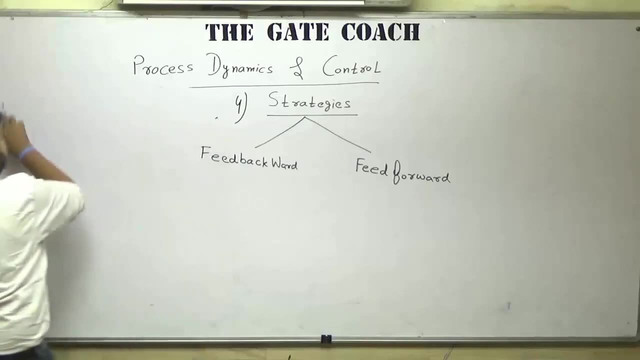 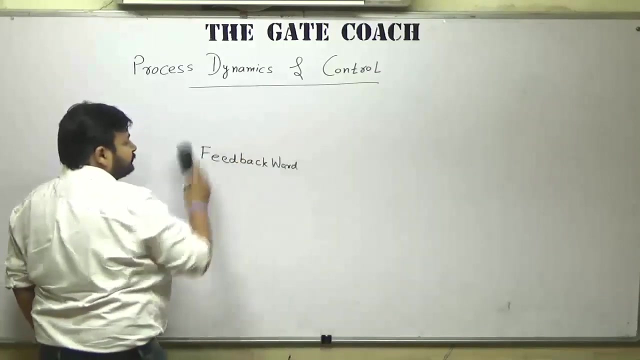 system becomes better and better and better. so we will discuss about both the strategies- feed backward and the feed forward- today. so first of all, as the name suggests here, feed backward. name: what comes to your mind first. something is going back. what comes in my mind first when i read this word is something that 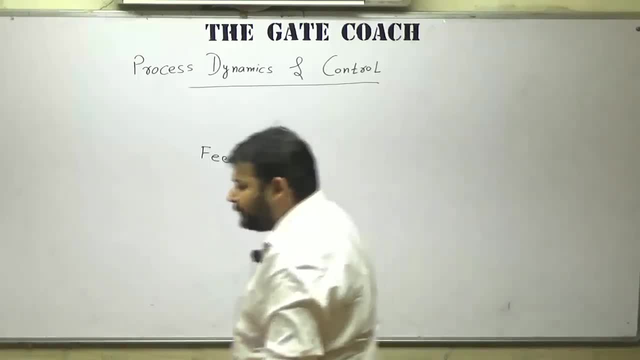 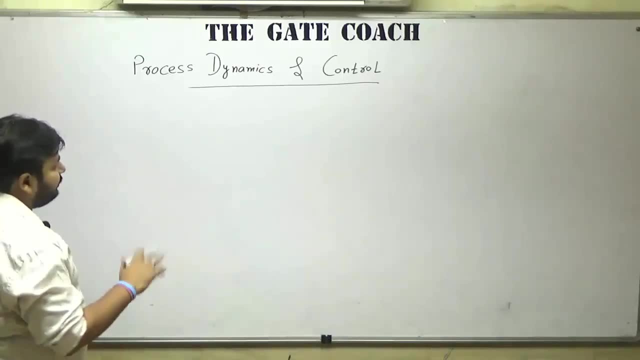 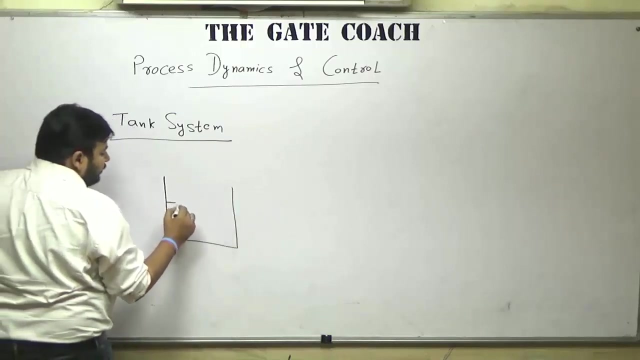 is going back. so if you recheck the block diagram then you will come to know that, yes, it is going like backward. so to understand the strategy, let us take a look at a tank system. that is the most used system in the case of control part. so in a tank system, this is a tank and let us say up to this. 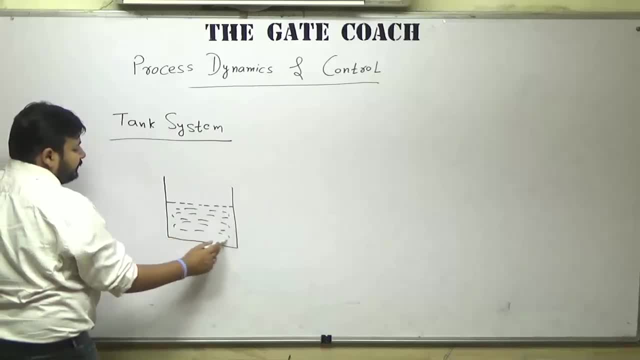 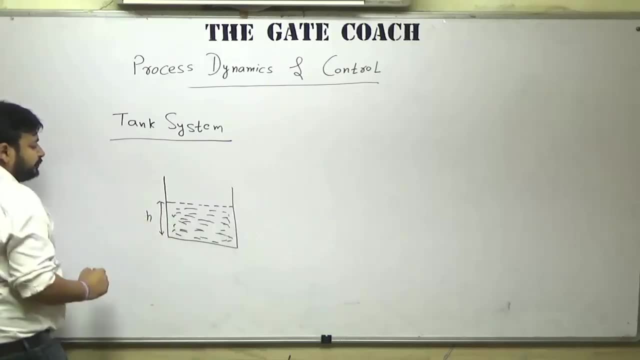 height. it is the liquid present. this is the height of the liquid level. let us say this height is small edge. now what is my aim of this tank system? the aim is to keep the height of the liquid level at hss, where ss represents steady state. so the aim of the system, 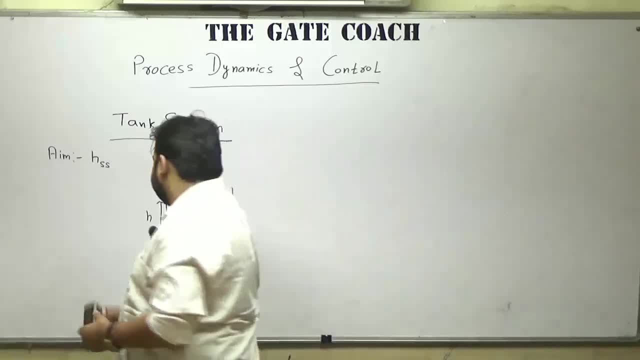 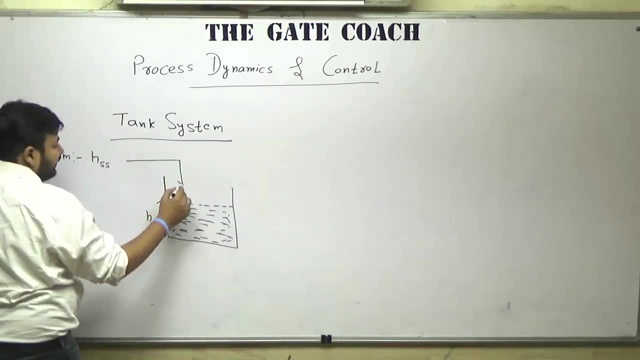 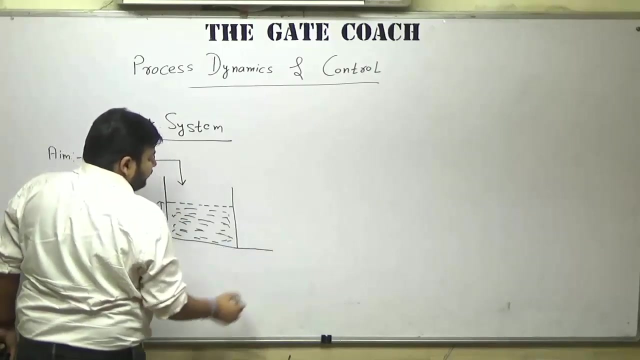 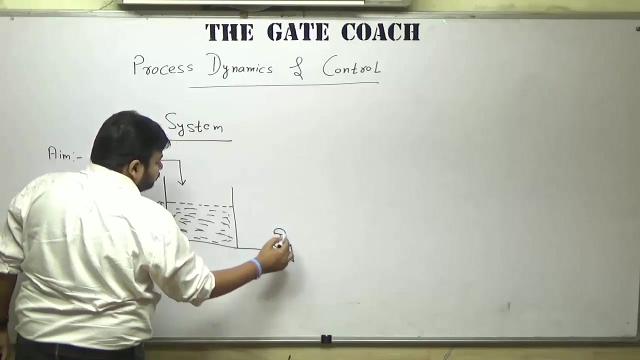 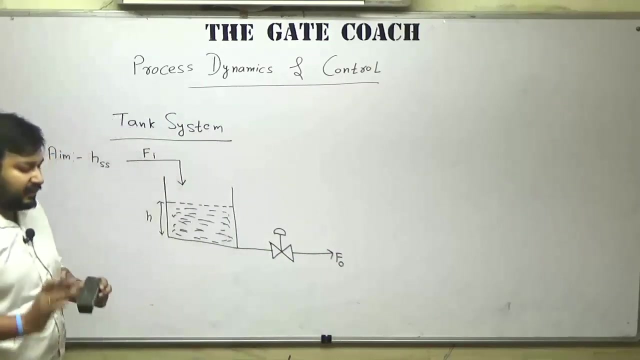 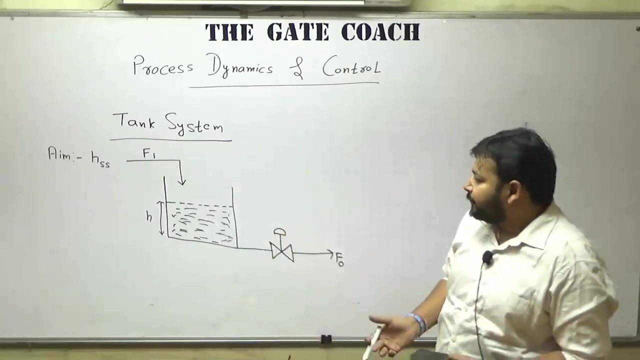 is to keep the liquid level at a steady state height. now there is an inlet and there is an outlet also, which is controlled with the help of a valve, and let us say that flow rate is f node. so that is a simplest tank diagram. some mass is coming in, some mass is going out, and there is accumulation of mass and 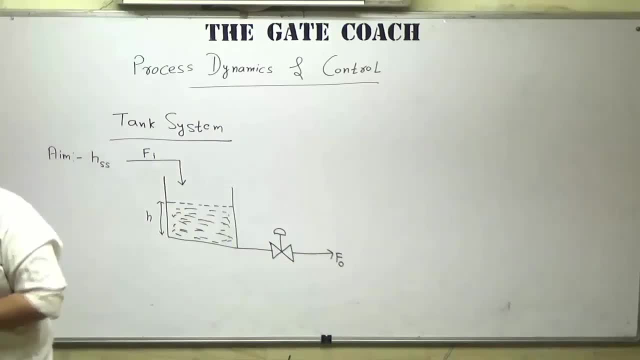 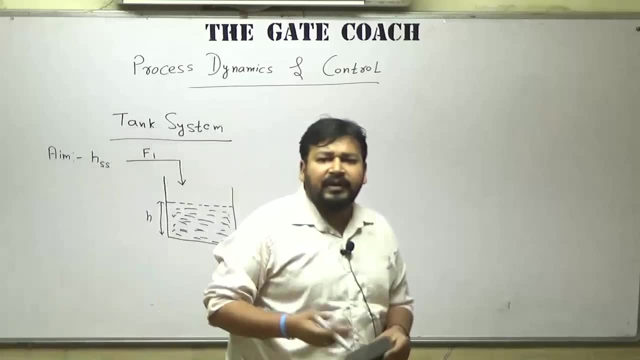 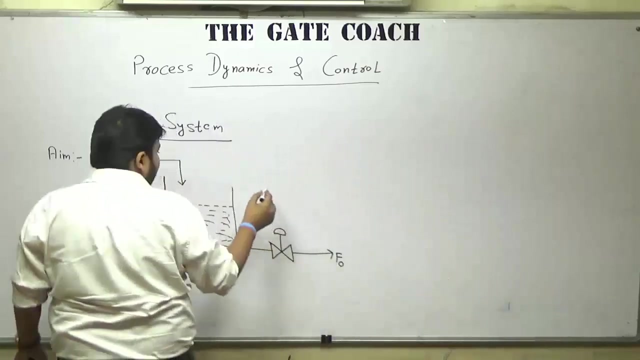 the height of this liquid level is h. and now what is my aim is to maintain the height at the steady state. so let us assume that i want to maintain the tank with this level controller. now, to fulfill my aim, what i need to do is to apply a control system. so let us assume that i 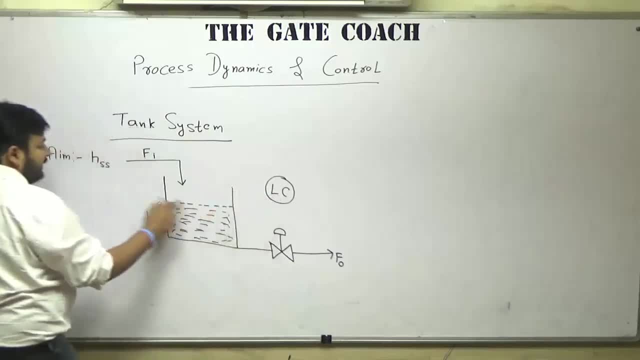 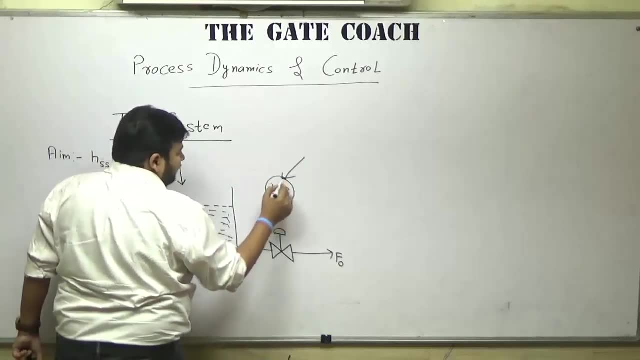 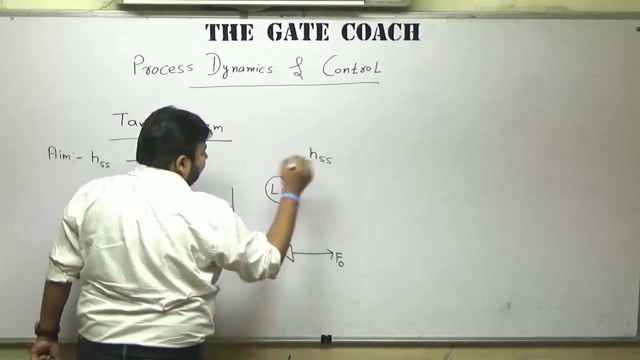 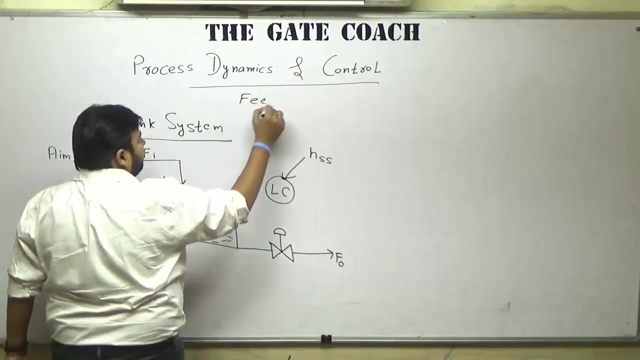 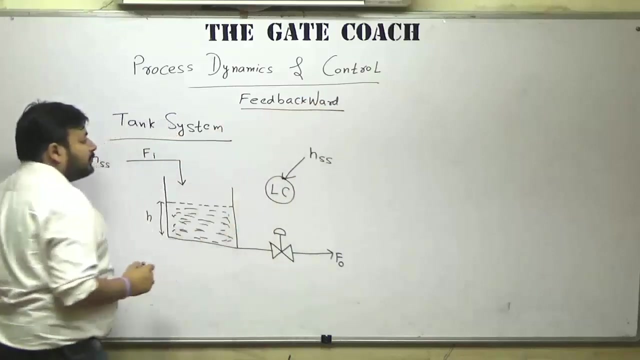 applied a level controller here whose purpose is to maintain this height at the steady state. so first of all, i need to tell this control system that at what height i want to maintain in the tank, so that height is h and hs1m. Now, in the case of feed backward, we are talking about feed backward. 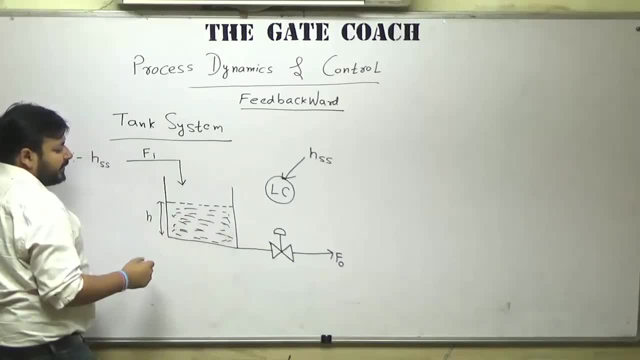 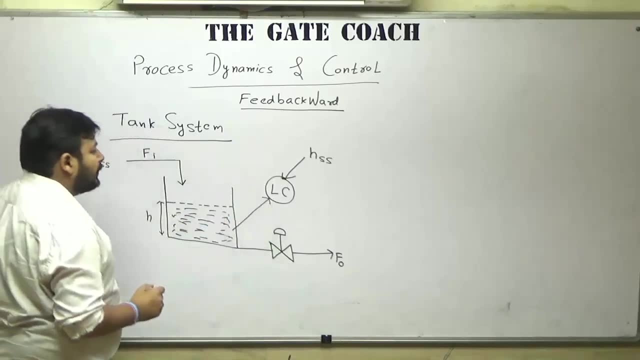 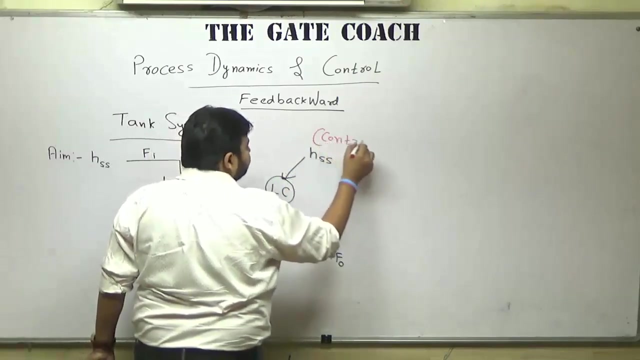 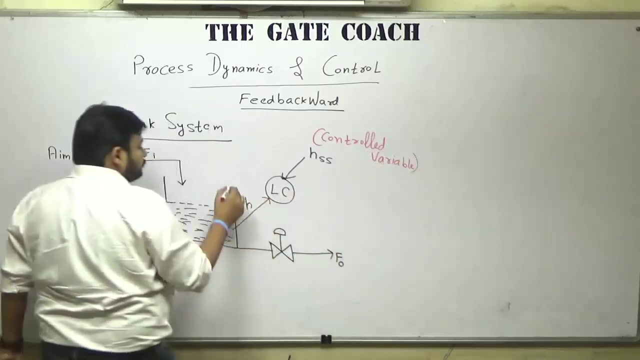 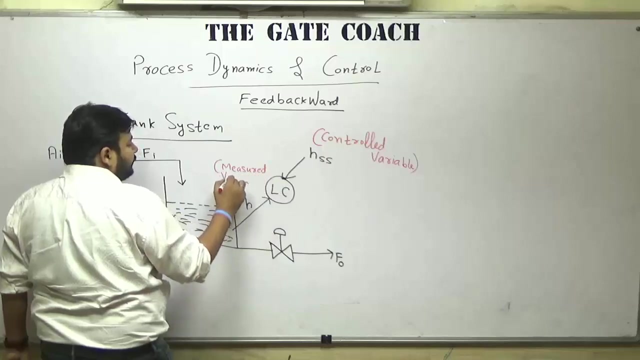 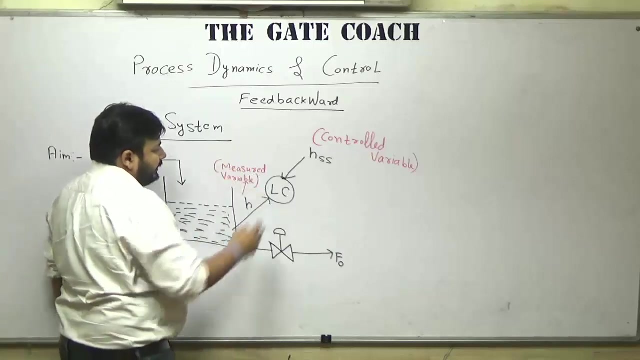 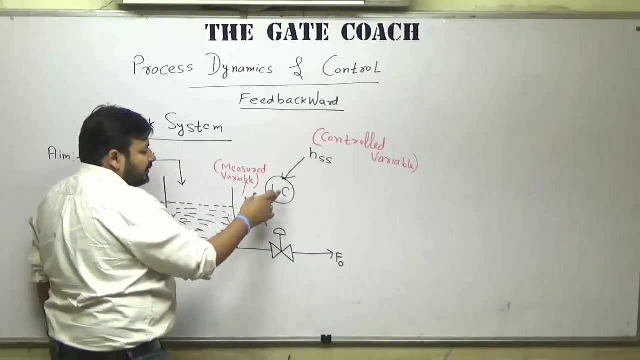 in the case of feed backward, whatever is the liquid level present in the tank that is measured. So this is H, So this becomes my controlled variable, This becomes my measured variable and after deciding the both, the comparator calculates the error. and to minimize that error, the controller will take its action. 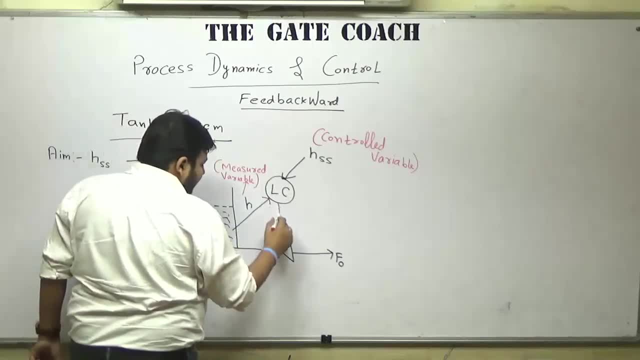 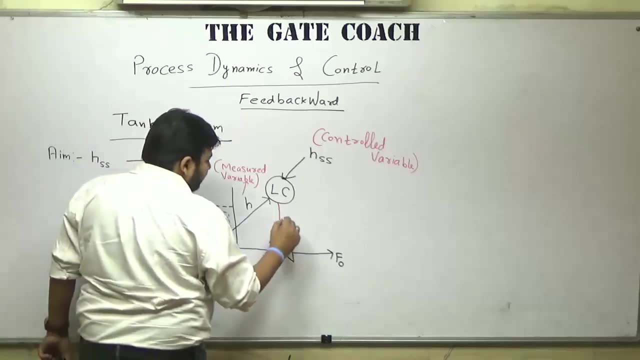 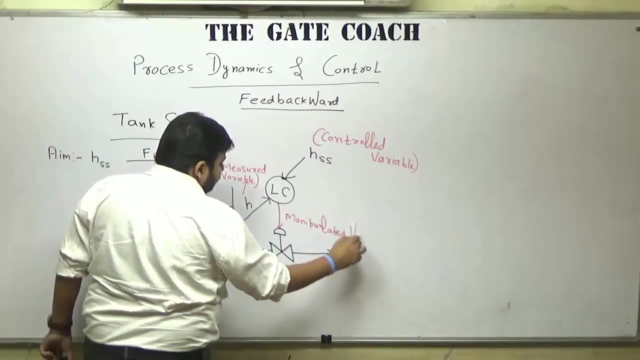 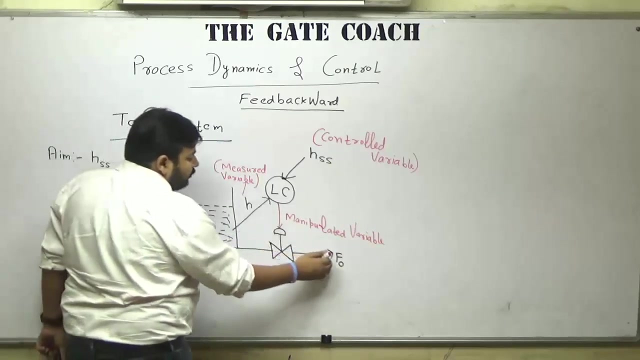 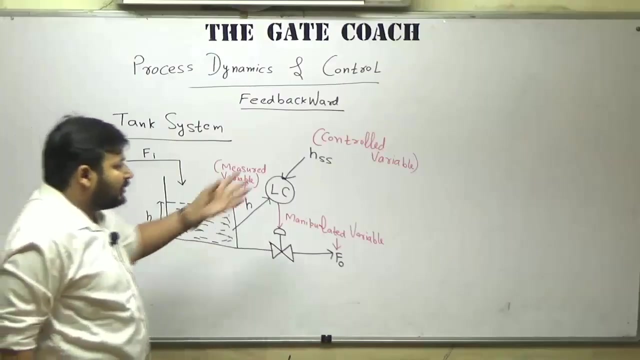 on the manipulated variable. And the manipulated variable here is valve. So here the valve action becomes the manipulated variable. So valve changes. what Valve changes? the outlet flow rate. So our manipulated variable becomes the outlet flow rate. So controlled variable is the one that we want to achieve. 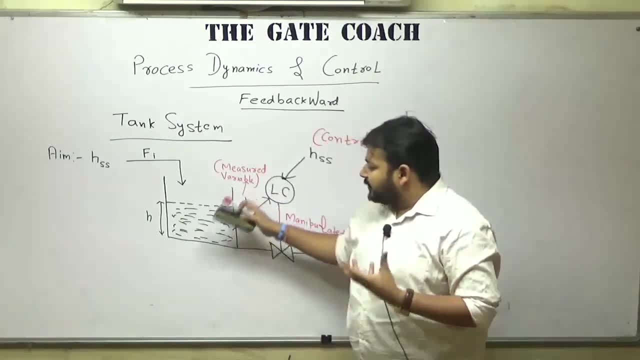 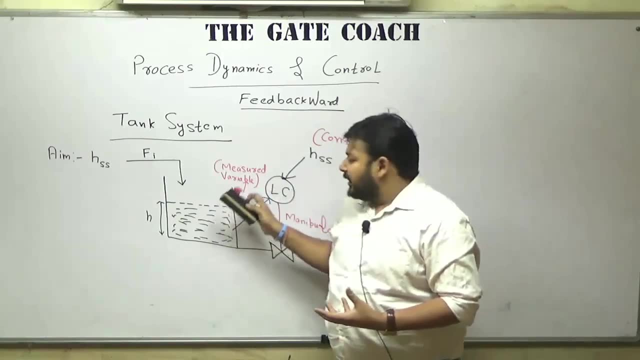 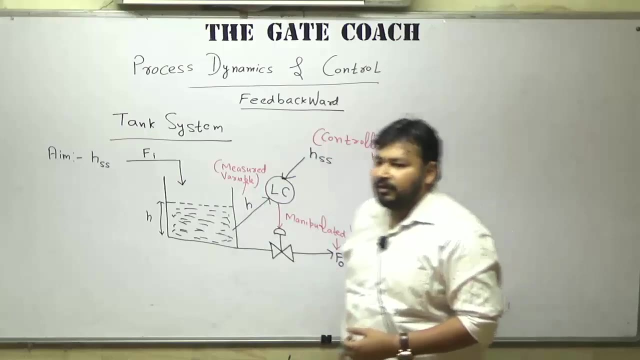 Measured variable is the one which is the present state of the system. This is the desired state of the system. This is the present state of the system. And to achieve the desired state, what variable needs to be changed? that becomes the manipulated. So by changing F node we can achieve the desired height of the liquid level in the tank. 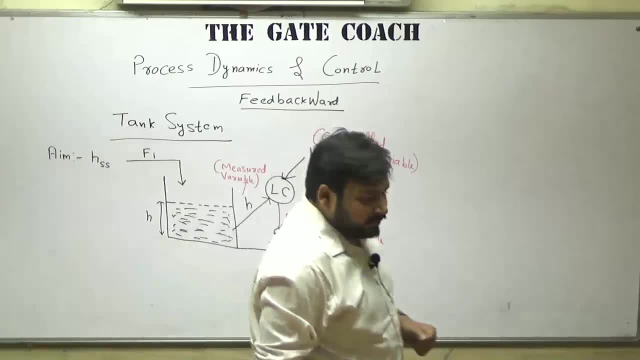 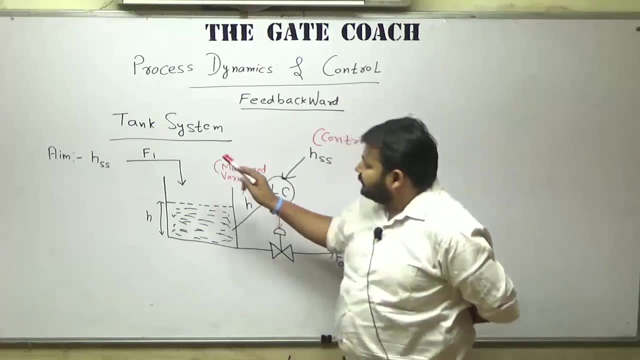 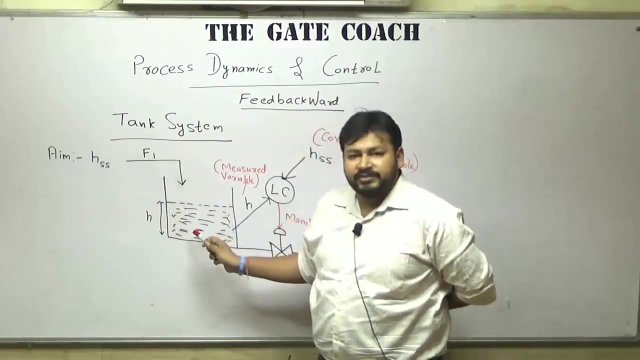 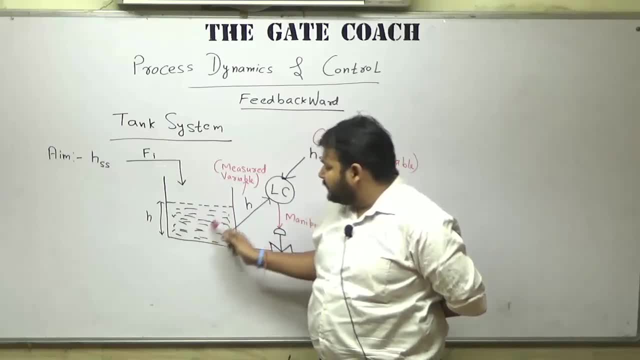 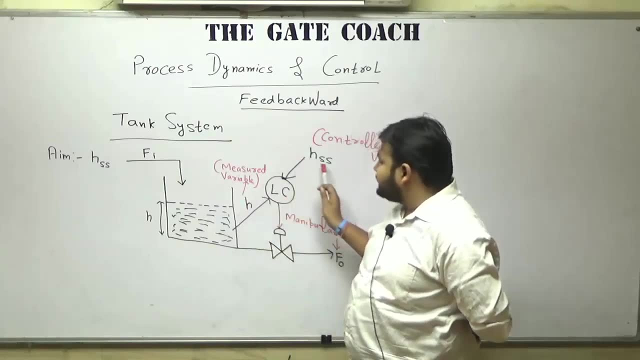 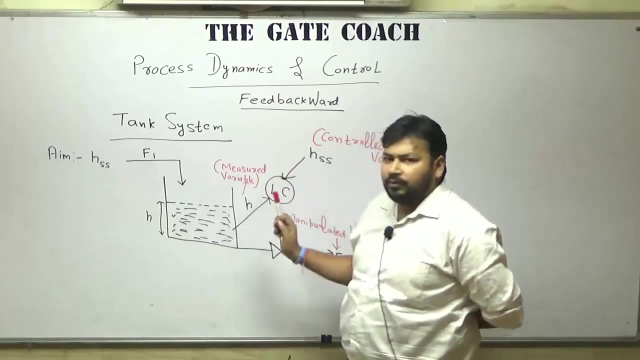 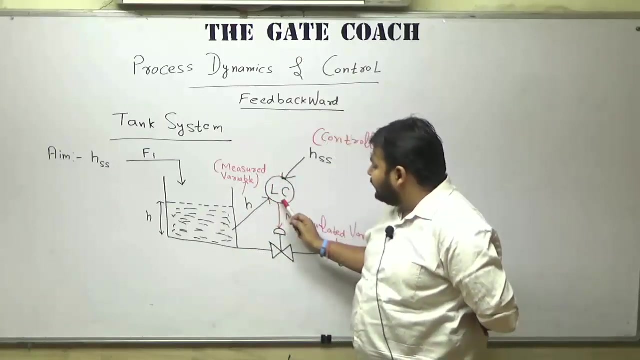 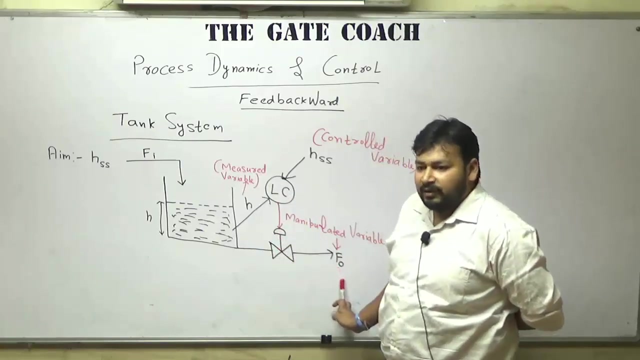 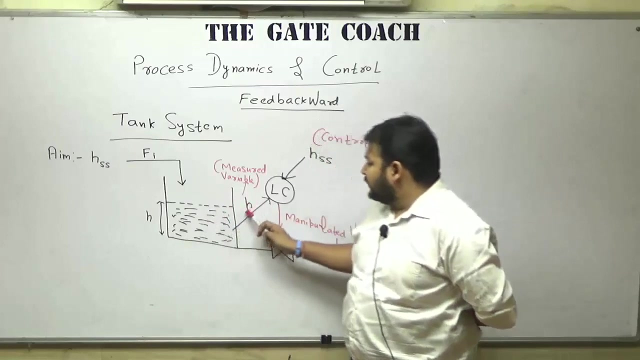 Now, as the liquid level in the tank changes, this H changes. As this H changes it is not same as HSS. now that means there is an error between the two. There is a difference, known zero difference between the two And that known zero difference is known as the error. Now controller will try to minimize that error by changing the valve opening, which in turn changes F node, that is, outlet flow rate. And as the outlet flow rate changes, the height in the tank changes again till the difference between the both becomes zero. 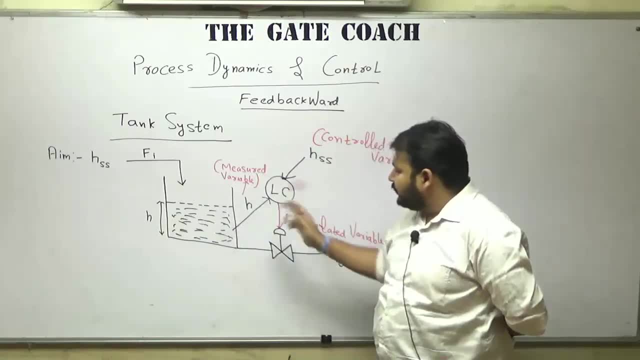 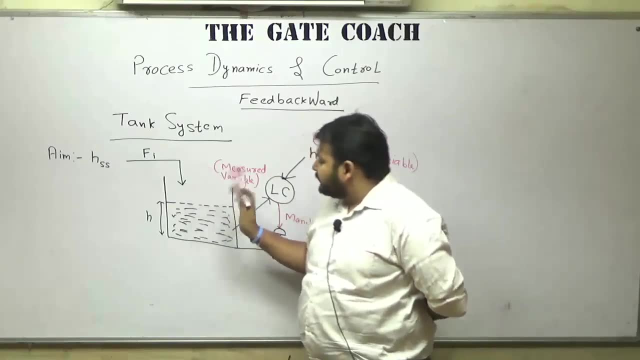 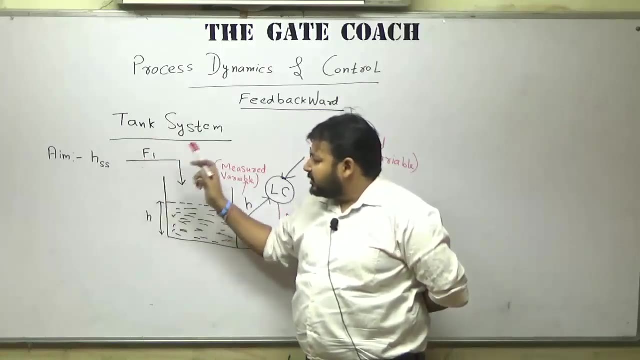 This is the control, how we are doing it. Now, in this whole scenario, one point to be noted: that if the system is at steady state, and at the steady state system, if there is any change in the inlet, that change will change the steady state of the system. 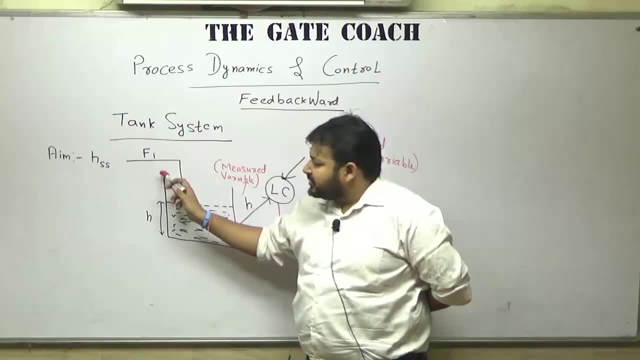 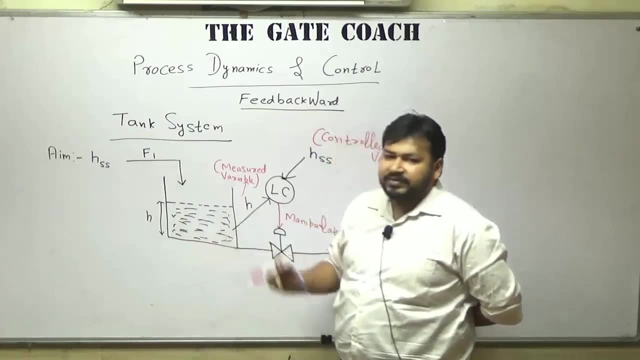 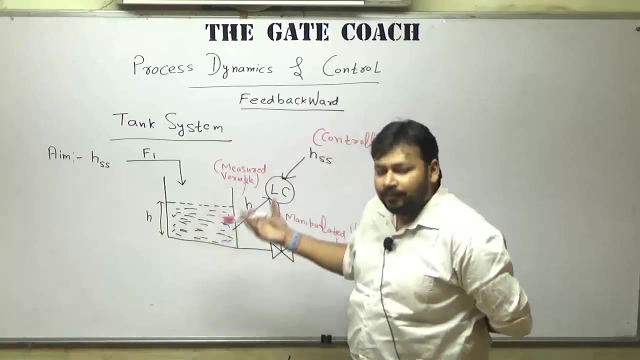 Or you can say the change in the surrounding, the change in the inlet, the change in the input will change the steady state of the system, Will disturb the steady state of the system And when the steady state disturbs then controller wakes up and try to regain that steady state again. 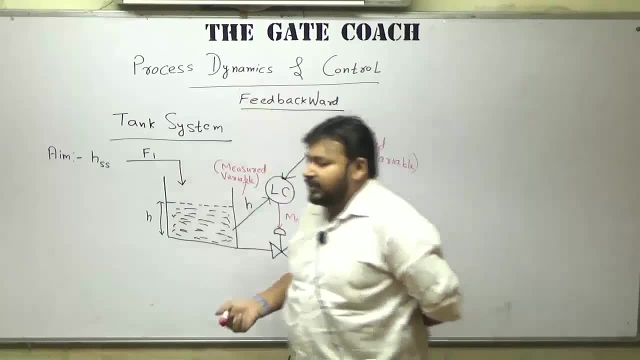 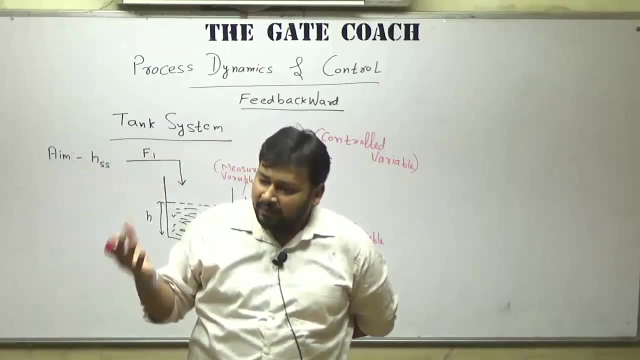 So that is known as the feed backward control strategy. That is a definition of the feed backward control strategy: That first of all, there is a change in the surrounding. Because of that change in the surrounding, the steady state changes. And when the steady state changes, after that the controller will try to minimize the error. 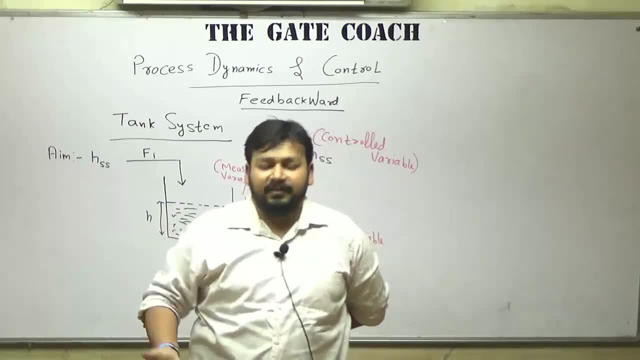 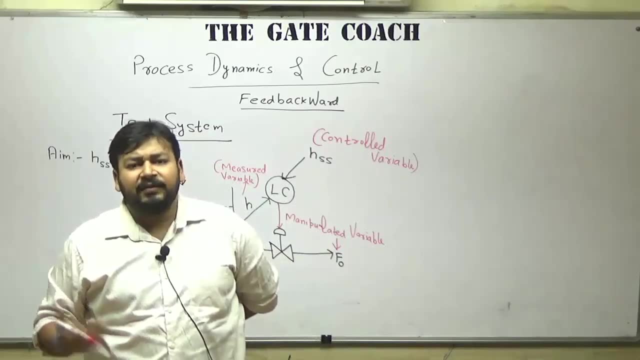 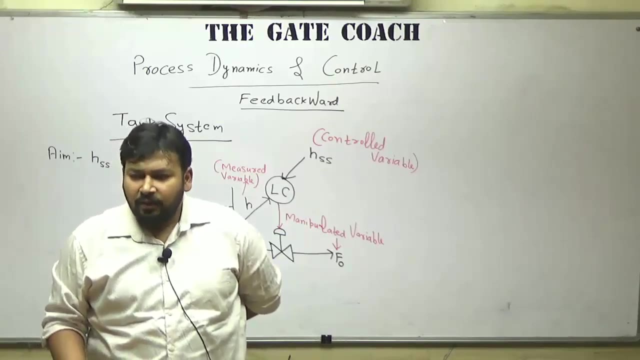 So the controller tries to regain that steady state again. This is known as feed backward control strategy. Like there are many examples in the real life also that are related to the feed backward, Like we are humans, Like all of you are preparing for gate or may be preparing for some interviews. 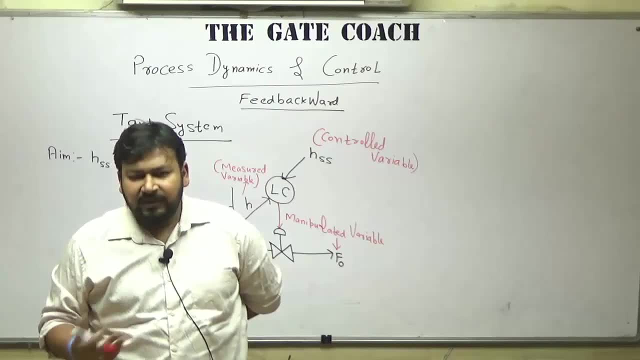 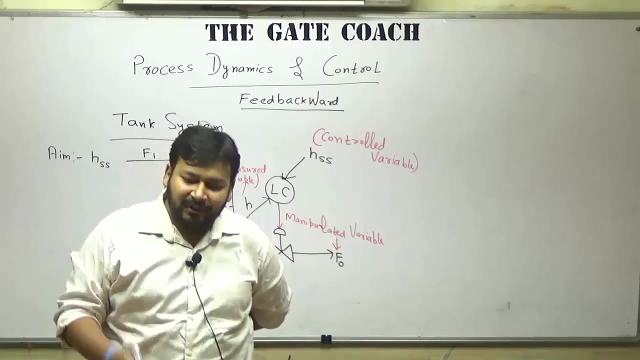 So, when the time is right, everyone, like teacher parents, say prepare, prepare, prepare, Give your 100%, give your 100%. But may be some of you don't give your 100%, don't prepare well and lose a chance to secure a seat in the MTech or in the PSU. 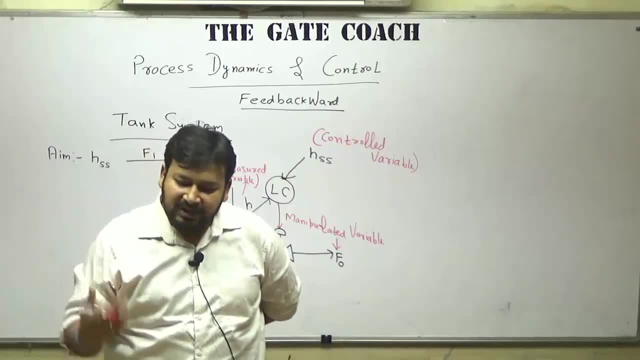 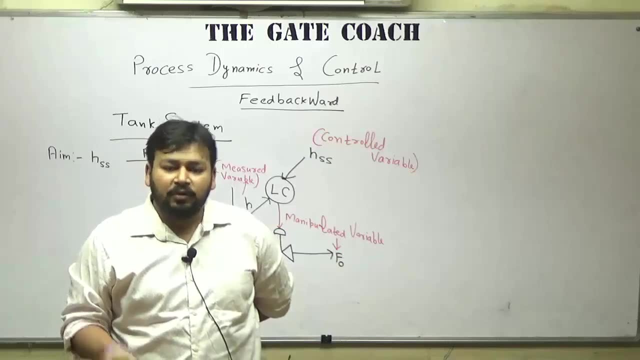 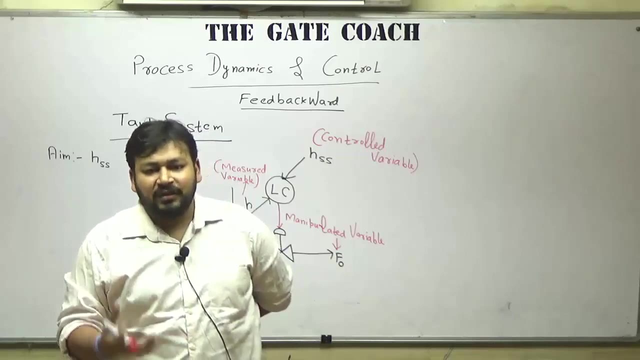 So what happens? that the change in the steady state takes place. That means, whatever you desire, you don't get it. Whatever you want, you don't get it. And when you don't get it, then your subconscious rises And then the subconscious will push you to do something. 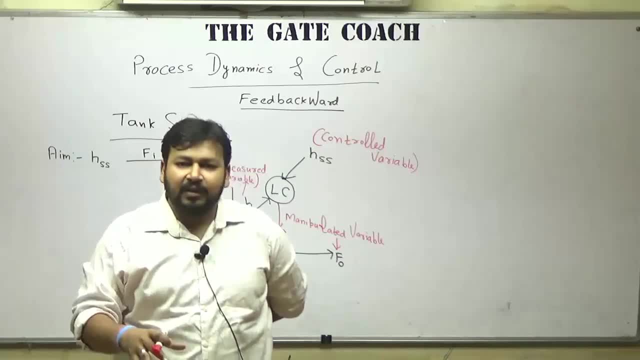 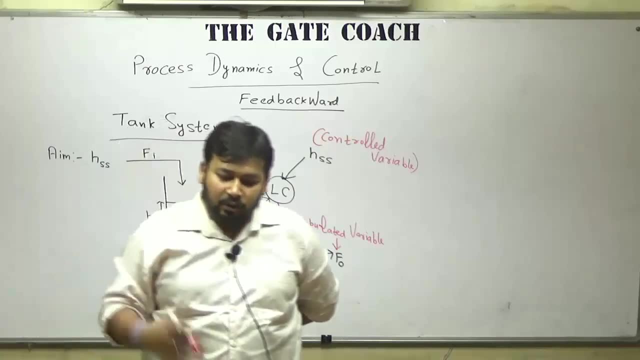 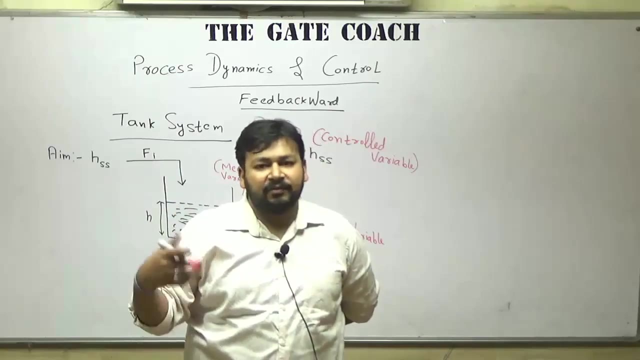 Push you to do it again, do it again, do it again And to get the desired target again. So, first of all, what is happening? that you are not putting your 100% effort to get the desired thing, And when the time vanish, when the time has gone, then you wakes up and tries to regain it again in the next year. 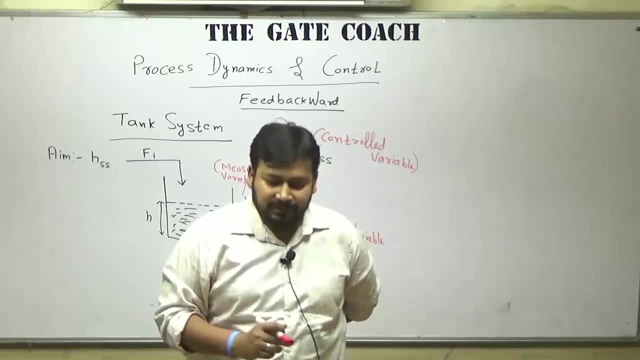 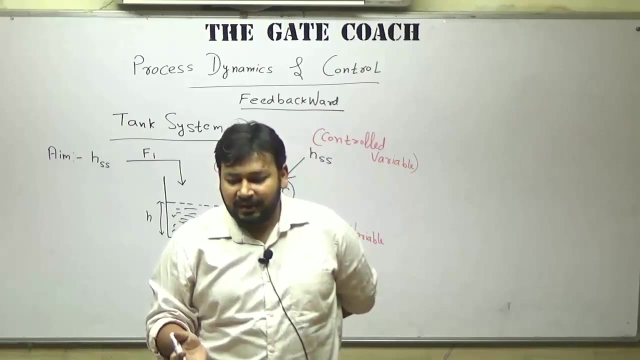 This is nothing but the feed backward control strategy. Like in our homes, Whenever the season changes, our parents suggest us to change our clothes accordingly. Let's say, from summer we are going to winter. There is a season change And there are most probable chances of suffering from cold cough fever or may be any other thing. 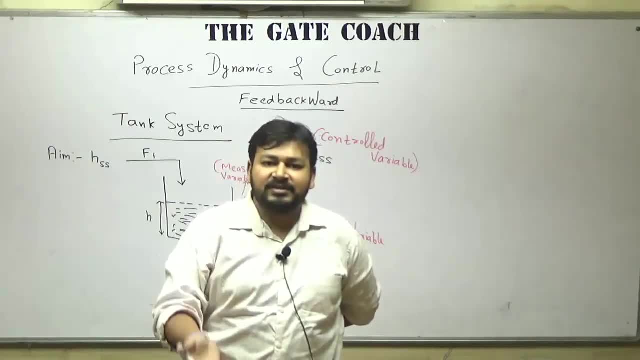 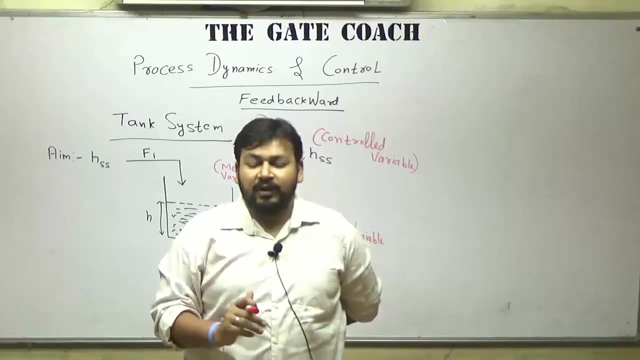 So in that point of time, the parents suggest that wear the clothes properly whenever you go out of the home. Now, some of you don't listen, And if you don't listen you get attacked by the atmosphere. And when you get attacked by the atmosphere then you take medicines. 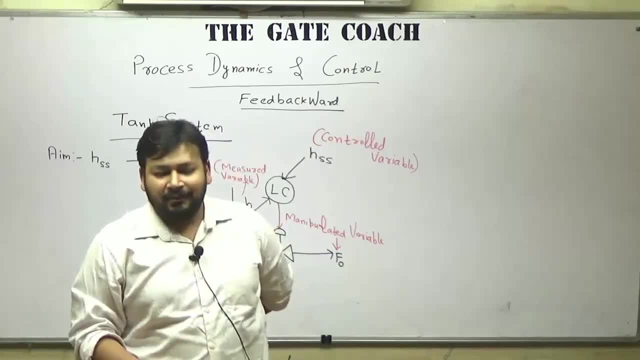 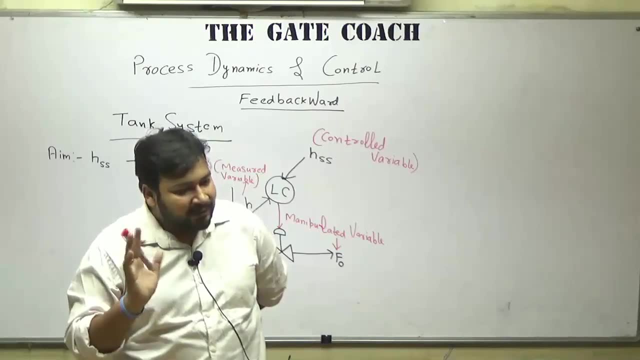 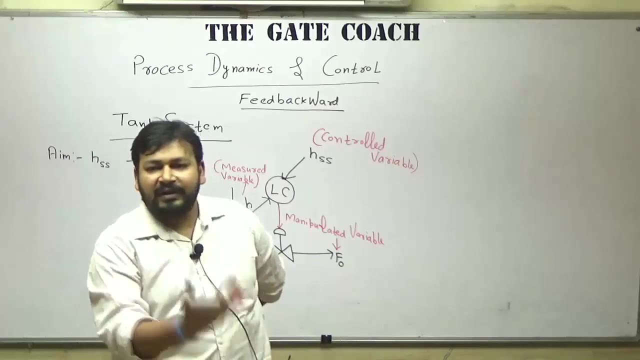 And try to be fit again. So what is in the initial point of time? Initially, you are fit, You are healthy, But you are not listening something. So if you are not listening to someone who is more experienced to you, What happens? the surrounding attacks. 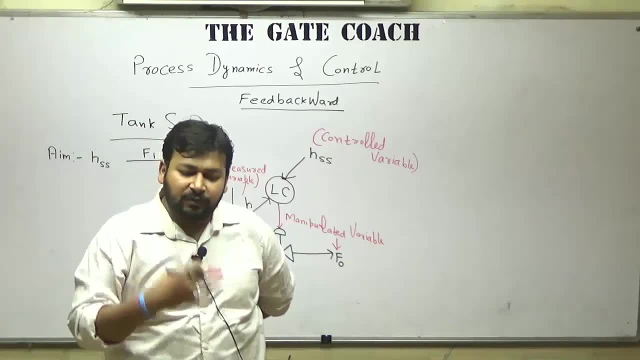 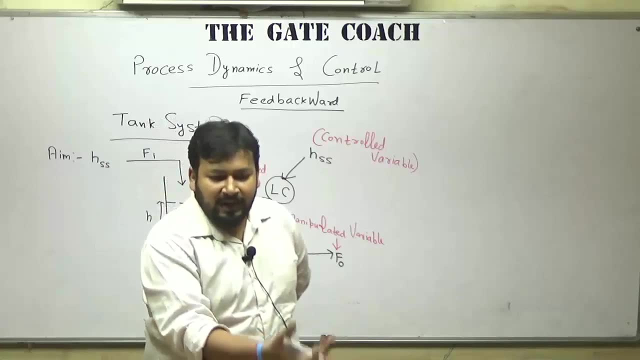 When the surrounding attacks The steady state of the body disturbs. Now, when the steady state of the body disturbs, Then by the external help, We are trying to regain our steady state again. We are trying to regain our steady state again. 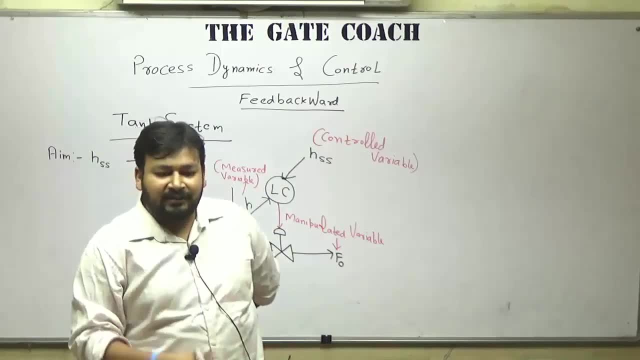 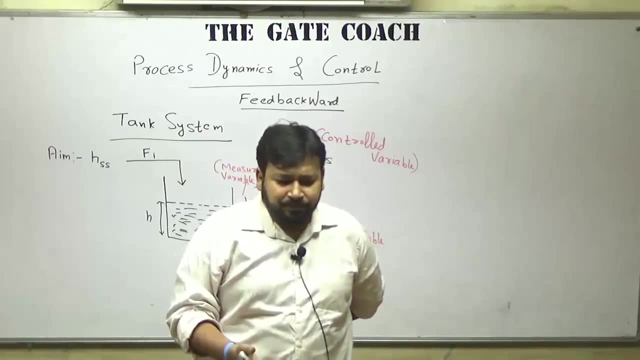 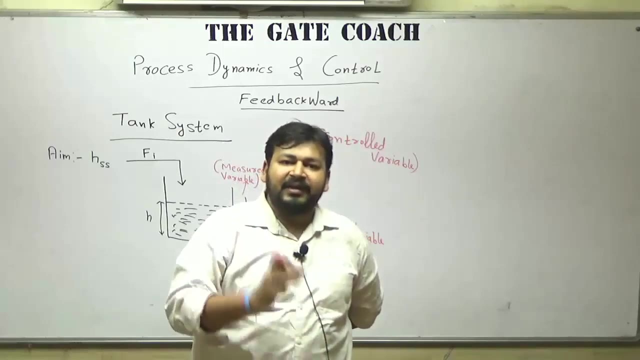 And same is happening here, That when the steady state of the tank, When the steady state of the tank is there Surrounding, comes, Disturbs the steady state, And now the tank is taking the external help from a controller To regain back its steady state. 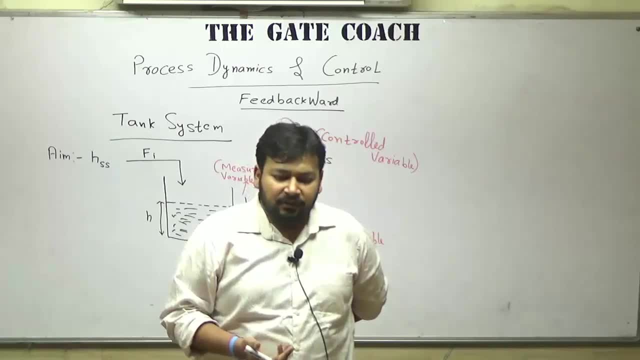 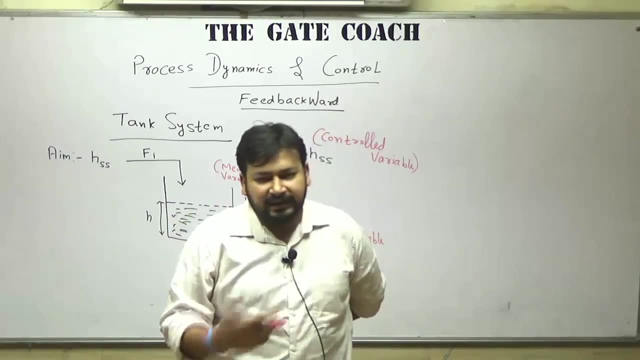 And same is happening with you guys. So there are numerous examples. So whenever We do not do The walk at the right time, The time will go, And after that time, if you do it, After that time, if you do the same thing. 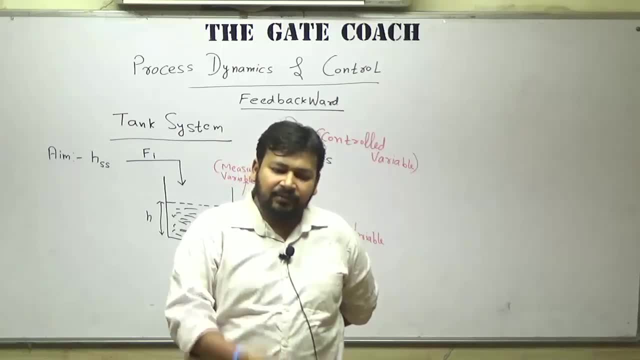 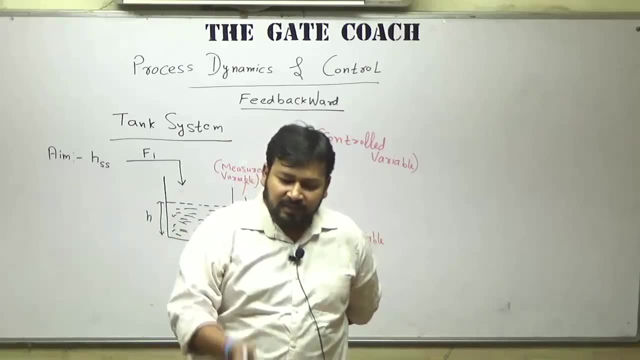 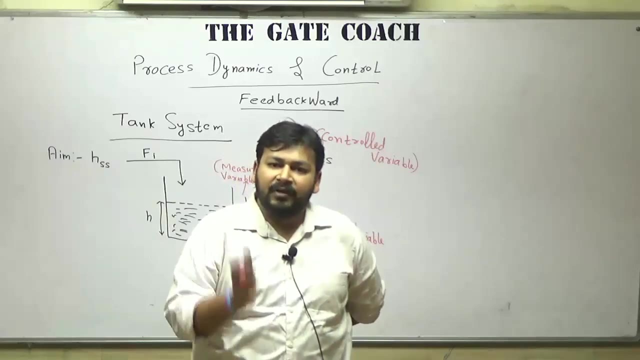 To achieve that thing, Then it comes under the category of Feed Backward control strategy. So, steady state is there, Something comes, Changes the steady state And now we are trying to regain the steady state back. This is feed backward control strategy. 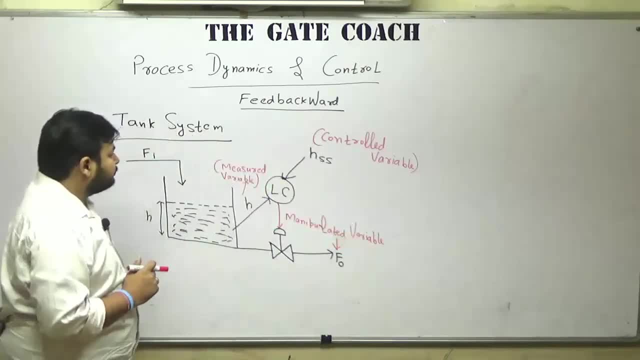 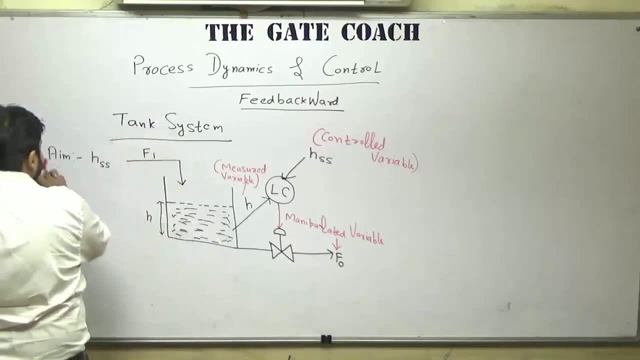 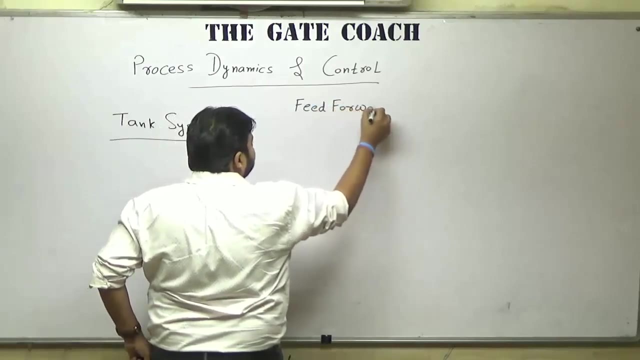 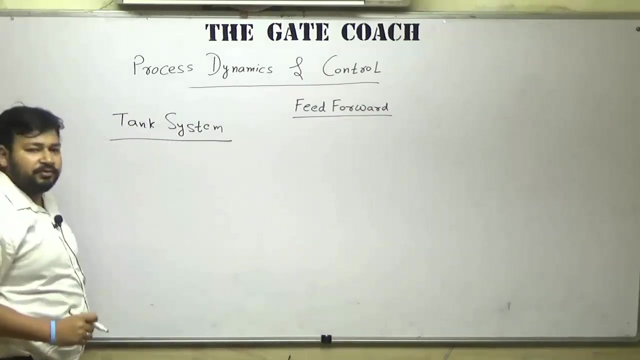 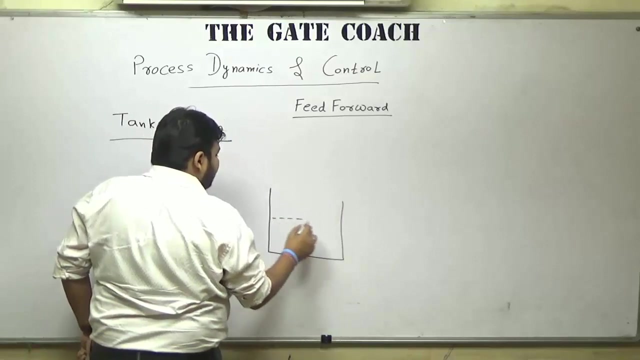 Like I explained in this diagram. I hope it is clear to all of you Now I will compare it with the feed forward also. Now here is feed forward control strategy. So again, we will take the help of tank system. This is the liquid level height. 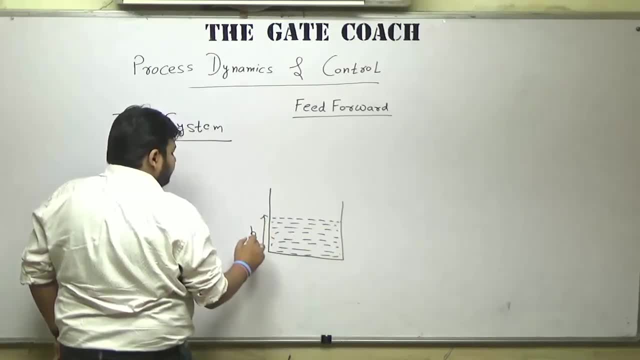 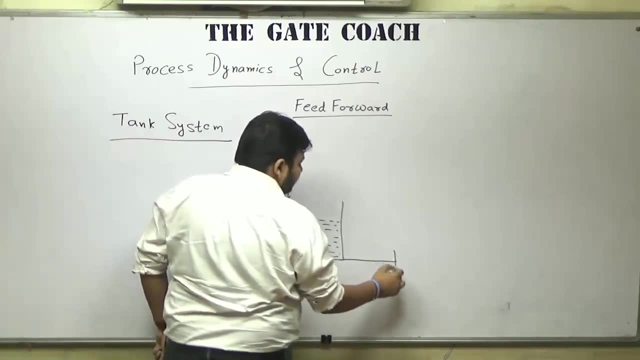 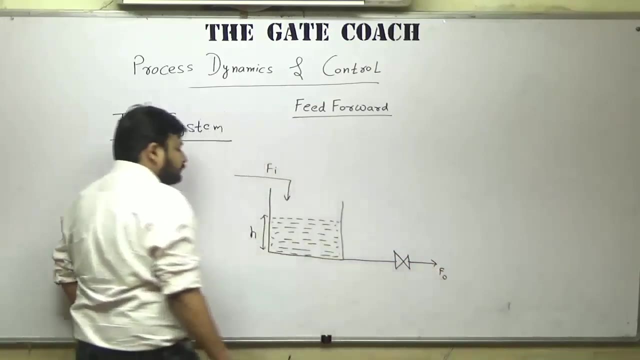 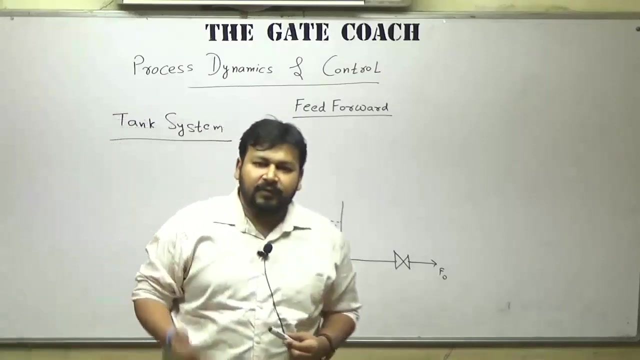 Let us say the height is H, There is some inlet And there is some outlet, Which is controlled with the help of a valve. Now feed forward. If I explain the feed forward first, Then feed forward is just the opposite case of feed backward. 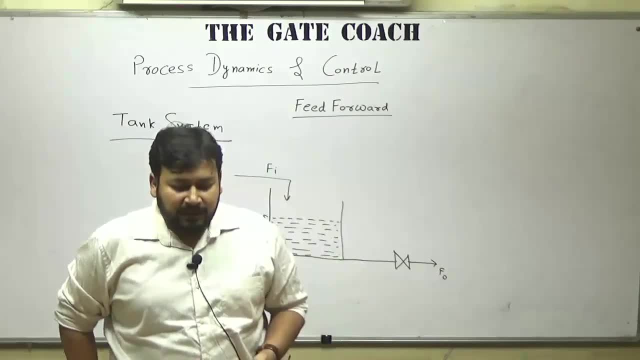 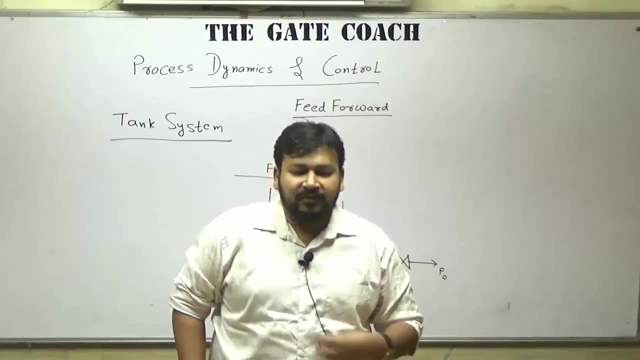 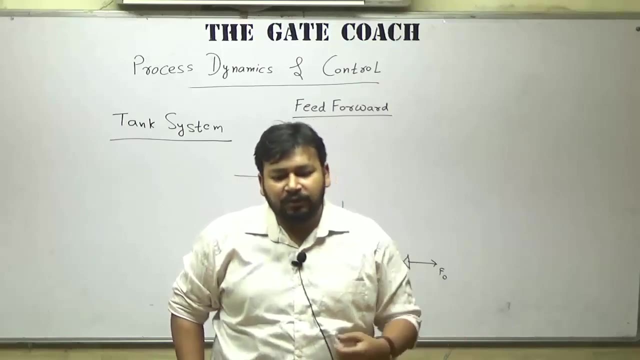 Now what is happening in the feed backward? That we are waiting for the time to finish. We are not doing anything, Or we are not doing sufficient Till that time, And when the time vanish, We wake up and do the things, But in the feed forward. 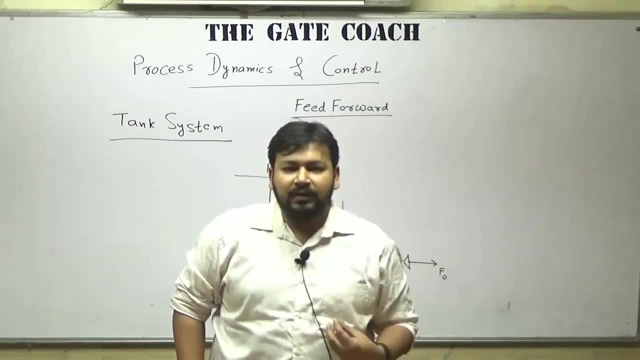 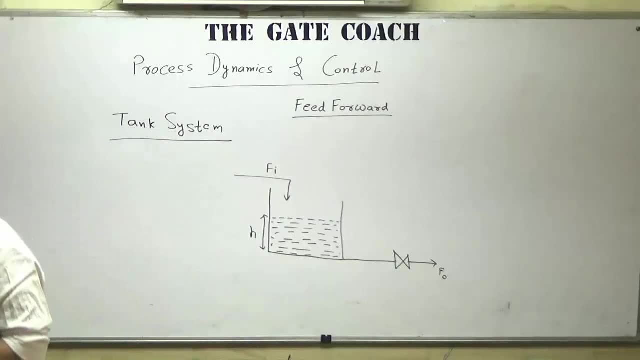 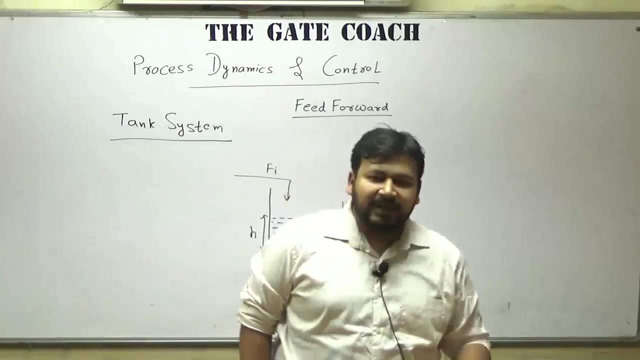 We are not waiting for the time to vanish. We are doing our best, We are doing sufficient, So we are doing whatever we can do And, after putting all our efforts Before the time, We get what we desired for. This is known as feed forward control strategy. 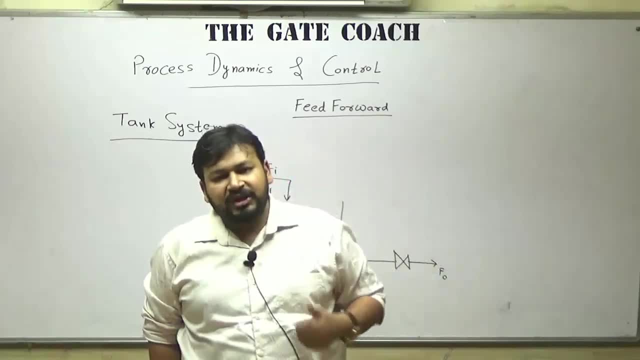 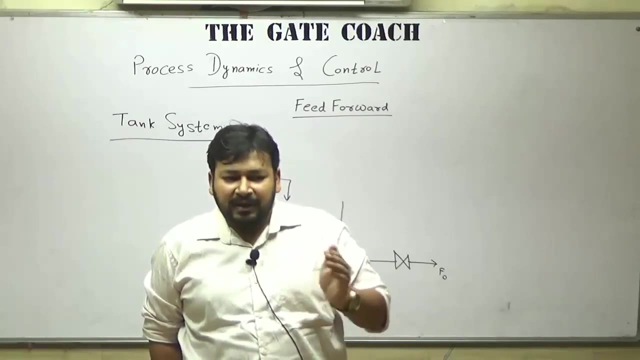 That means now Surrounding cannot change our steady state of the system. Before it enters the system, The controller will try to prepare the system accordingly. So that means whenever the season changes, Parents suggest to change our pattern of the clothes, And if we follow, 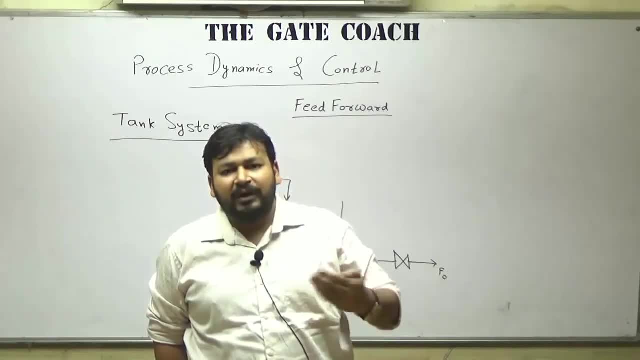 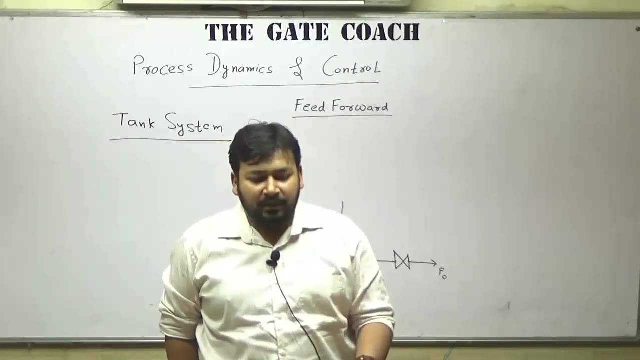 Then it will be very hard For the atmosphere to attack us. If we listen to our teachers, If we listen to our instructors And follow them, Then it will be very sure To get a success Or to secure a seat In the MTech or in the PSU's. 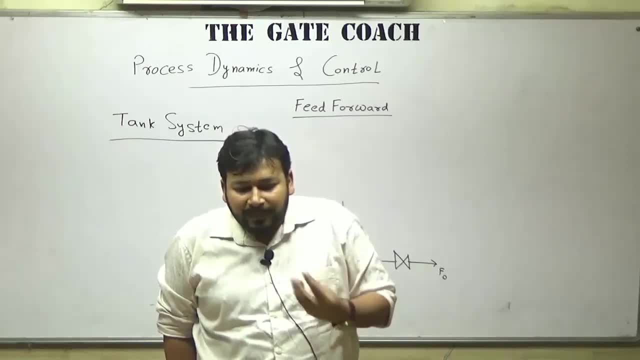 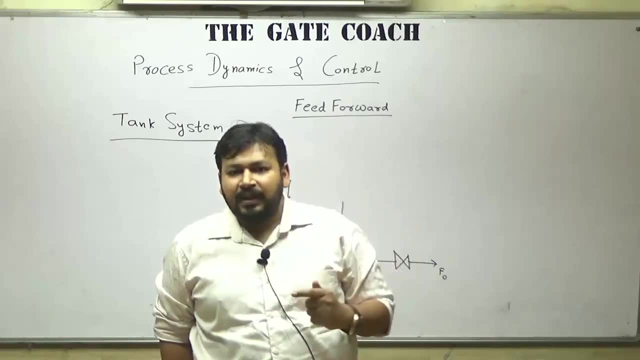 So it's just about to follow And to prepare ourselves For the next challenge. So if we know That in our life The challenge will gonna come, And if we prepare ourselves for that challenge, Then for sure, Then for sure. 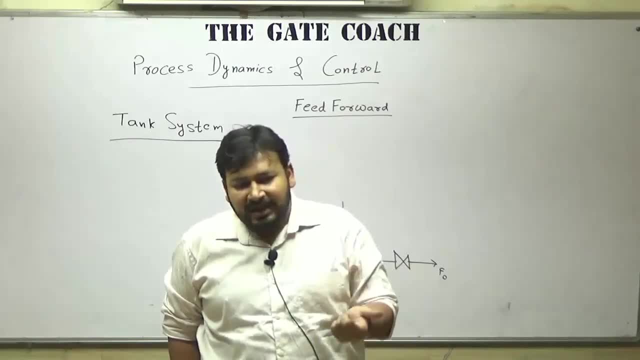 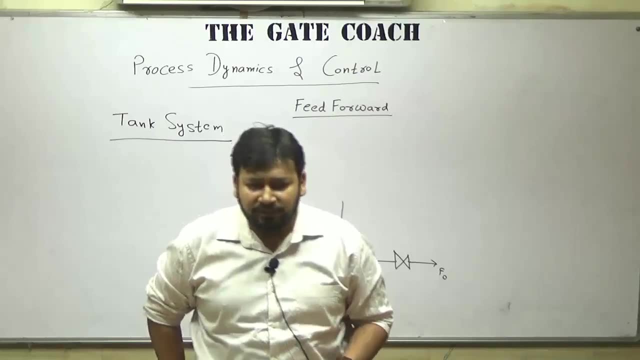 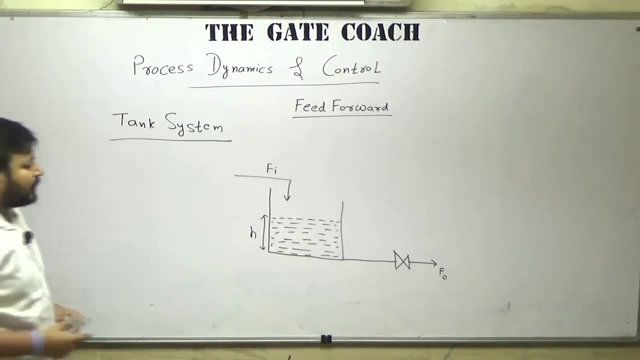 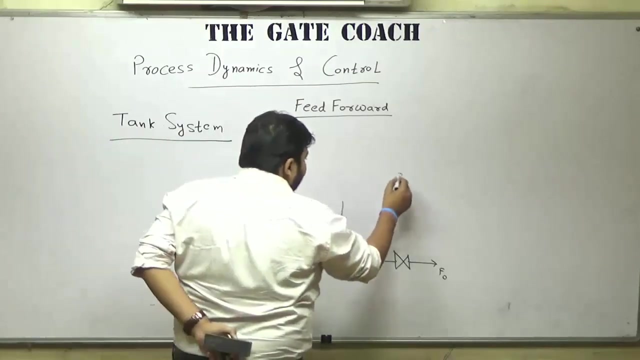 Then we can fight against that challenge, And that challenge will not harm us, That challenge will not affect us. So this is known as feed forward control strategy. Now to understand this feed forward control strategy: In the tank system, Again, we use the level controller. 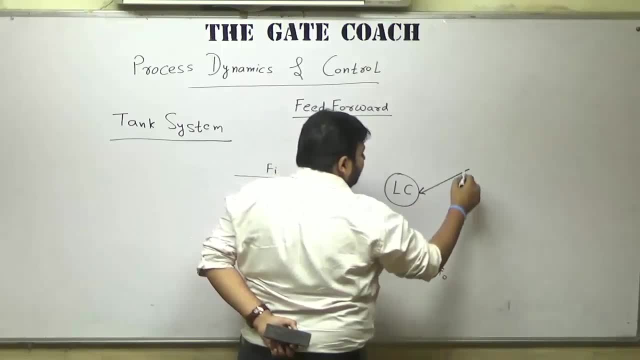 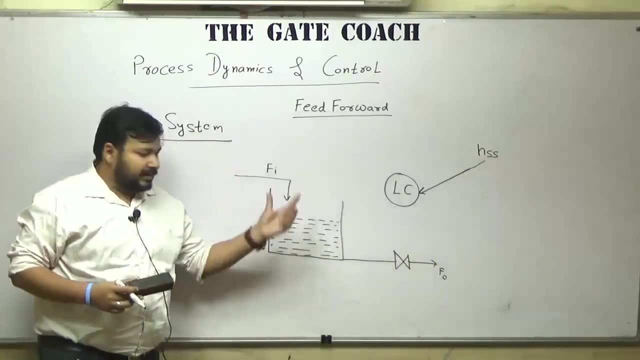 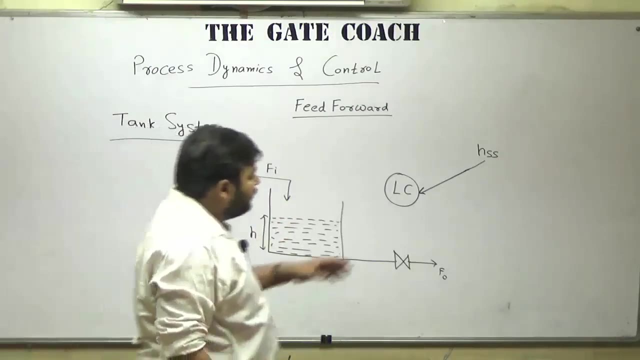 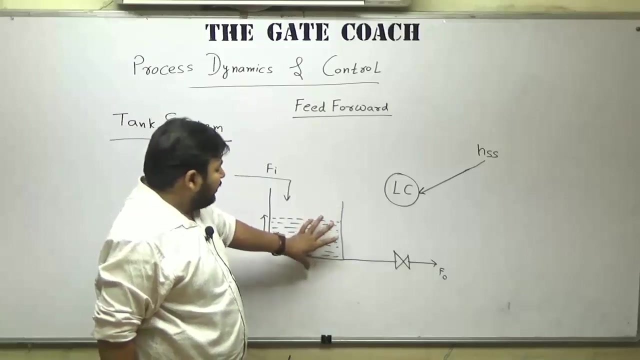 And we need to tell the level controller That what is our desired height That we need to maintain in the tank Now, in the feed forward control strategy, To maintain this height? We are not looking for the present state of the system, We are not looking out for it. 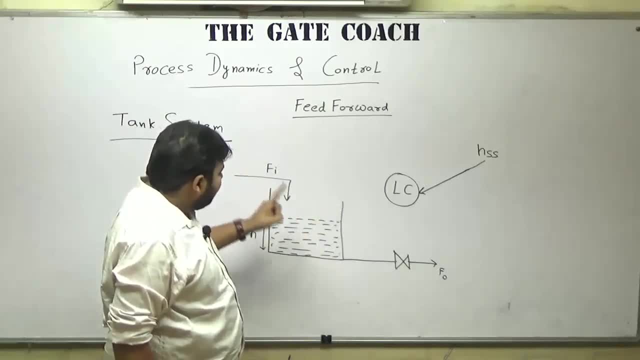 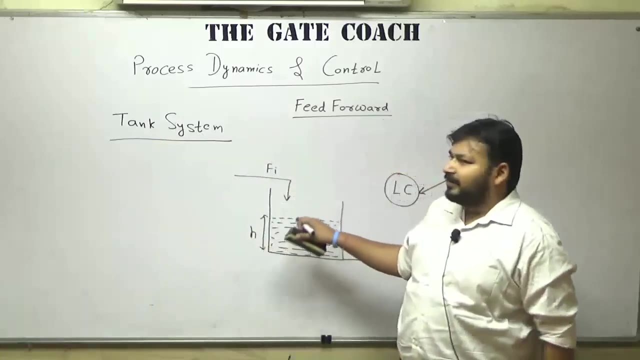 Our main aim that When this disturbance enters the system, The system is ready to balance that change. So let's say, if the inlet is more, The flow rate is more, Already the level of the liquid in the tank is less, So that when this stream enters the tank, 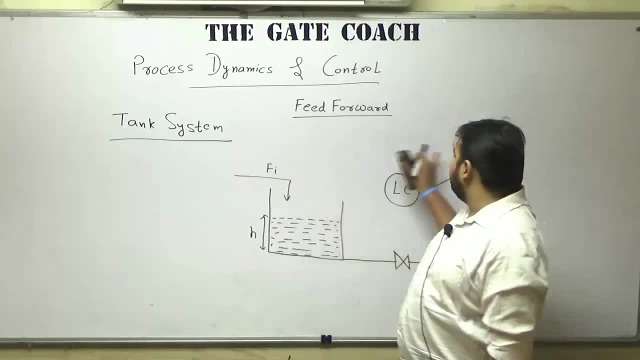 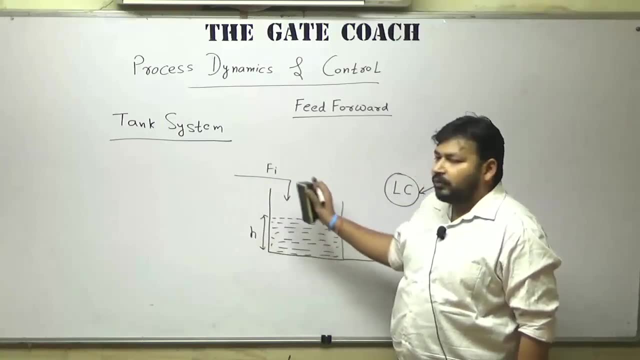 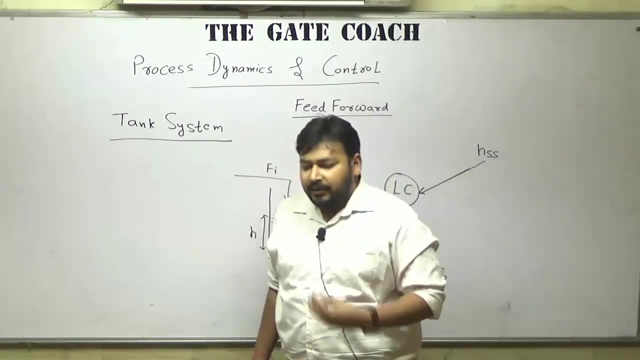 The overall height comes out to be equal to HSS, And if the flow rate is less, The level should be more, So that the overall height again should be equal to HSS. So, in this strategy, what is our main aim? Our main aim is to prepare the system. 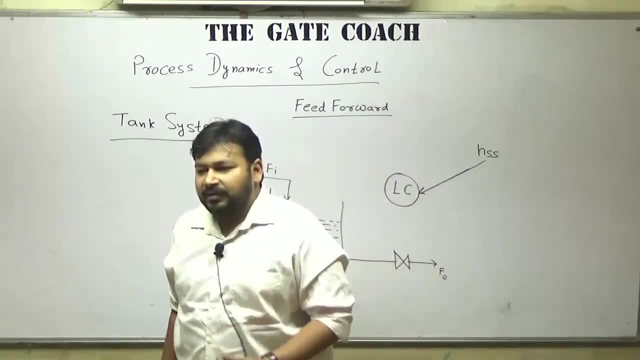 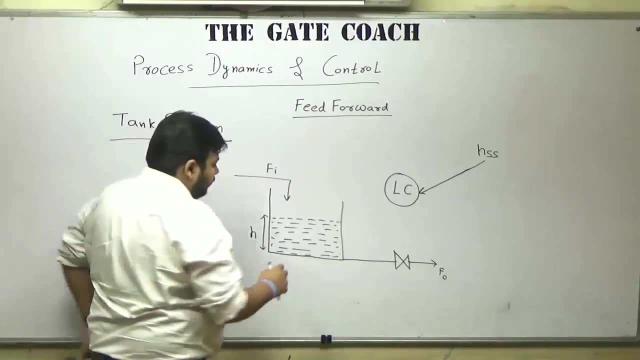 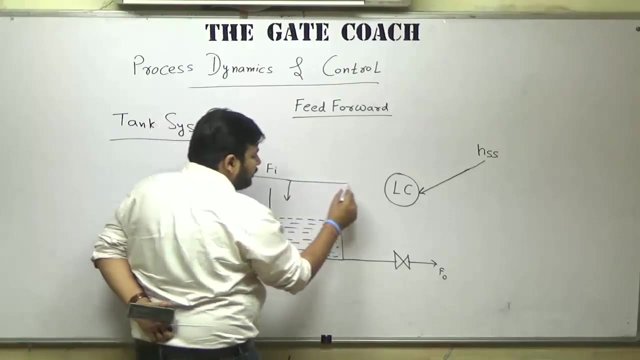 According to the disturbance, Is to prepare the system According to the change in the input. So now, instead of measuring The height of the liquid level, What we will do, We will measure the, That is, the difference between the feed backward. 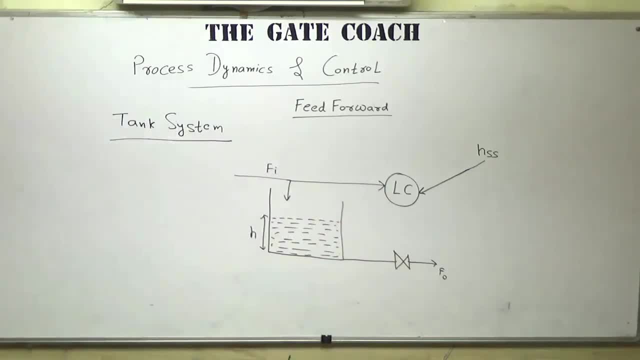 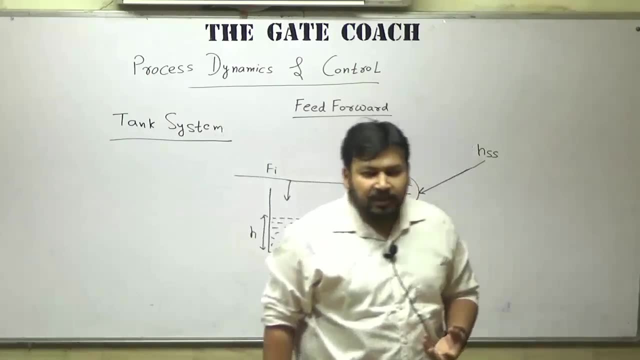 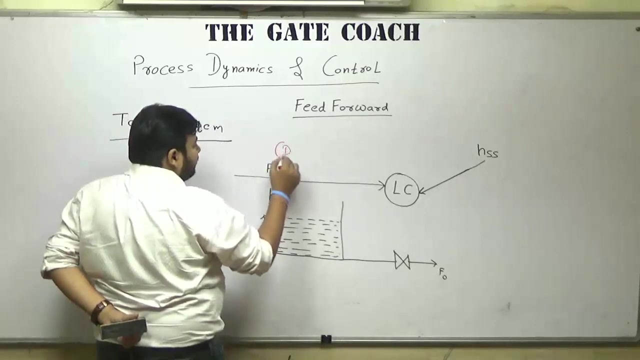 And the feed forward control strategy. That feed backward control strategy We will measure the present state of the system, While in the feed forward control strategy We measure the change in the input or the disturbance. So we can say this as the disturbance. 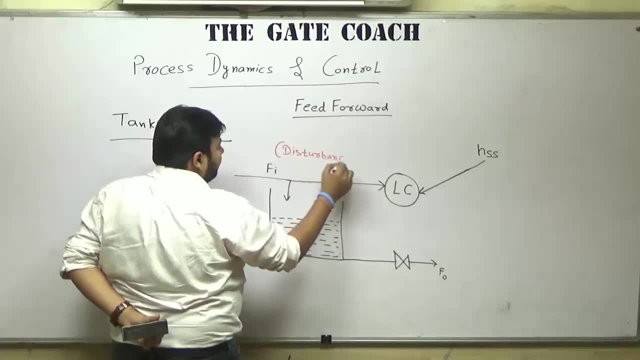 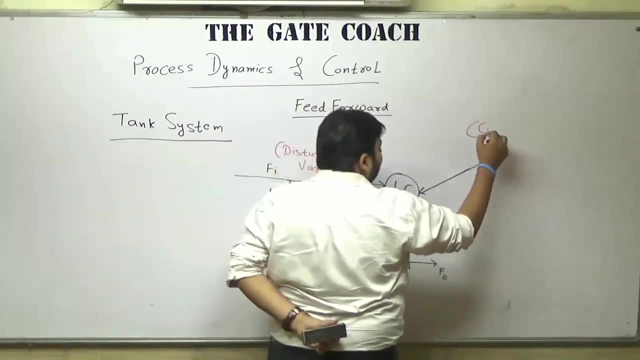 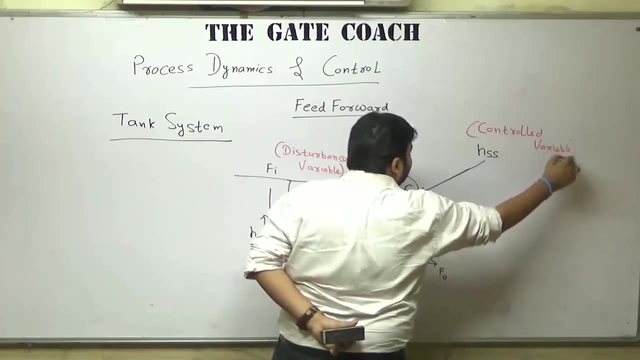 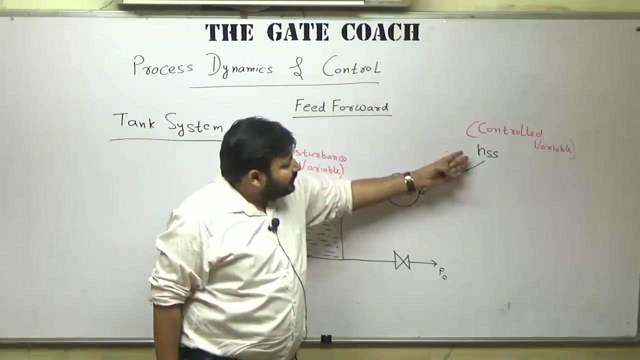 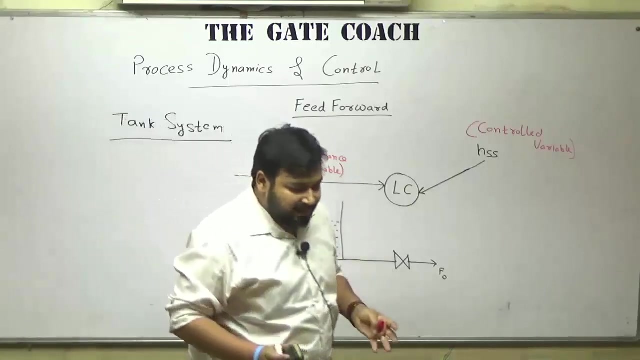 Disturbance variable And this one is the, again the same, That is, controlled variable. Now, one very important point to note here: that This control variable is in terms of height And this disturbance variable is in terms of flow rate. So when both the data enters the comparator. 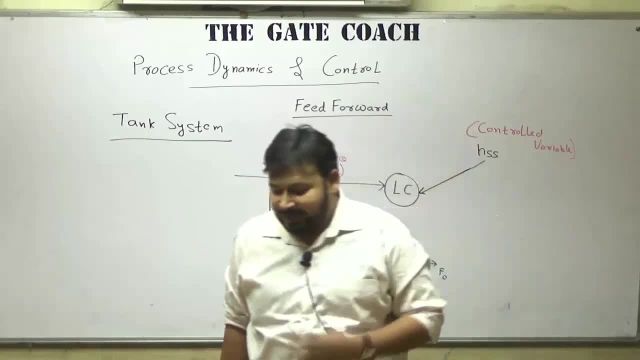 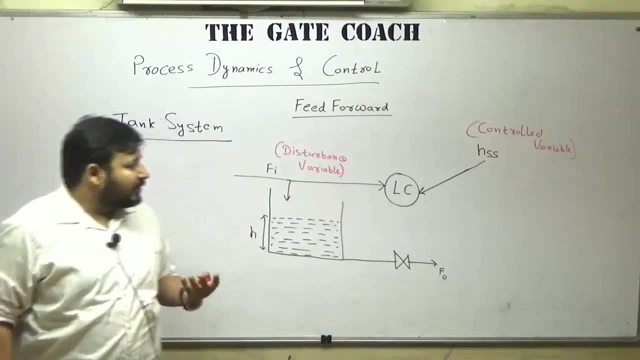 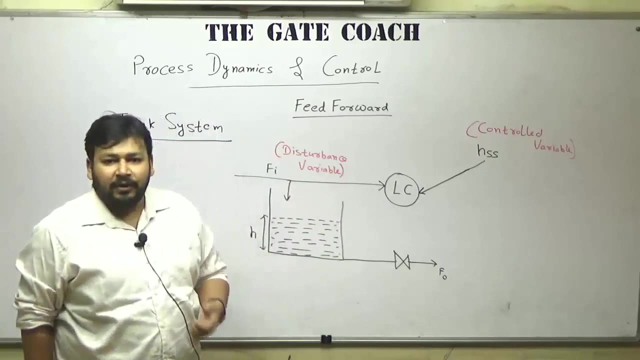 They cannot be supplied. They cannot be subtracted, Because for the addition And the subtraction The variables must have the same units. The variable must be of same nature. We cannot subtract meter with Some meter cube per second. We cannot do that. 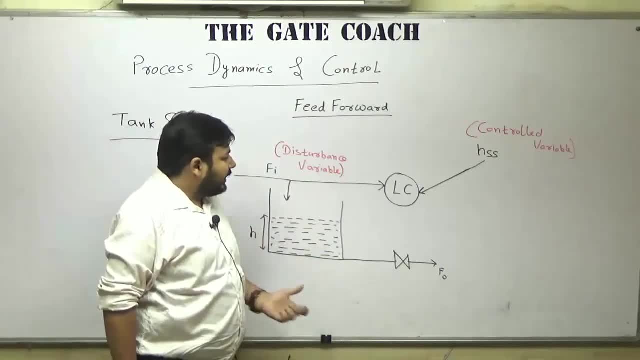 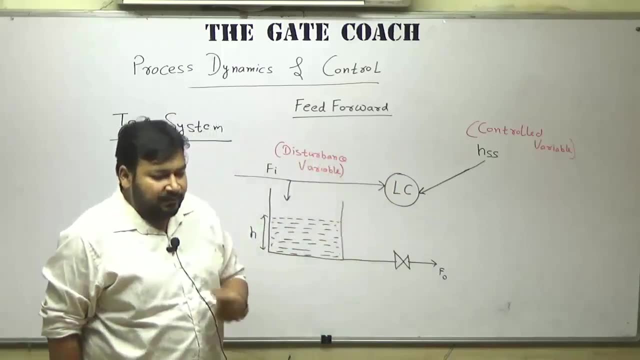 So what we need to do here We need to change. Either we need to change flow rate into height Or we need to change height into the flow rate. So for that, what we need, We need a Model. again, That is not needed in the feed backward. 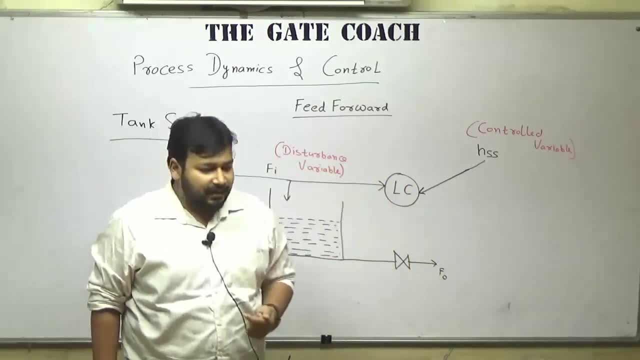 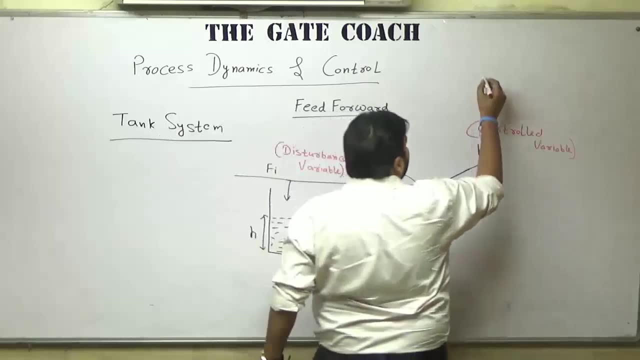 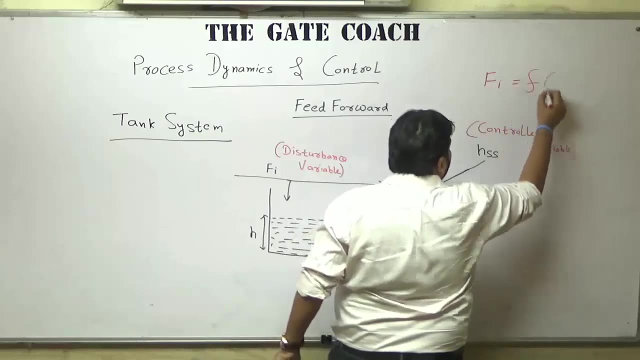 But in the case of feed forward, We need it So that we can change Height according to the flow rate Or flow rate according to the height. So what we require here? We require a Relation Between The inlet flow rate. 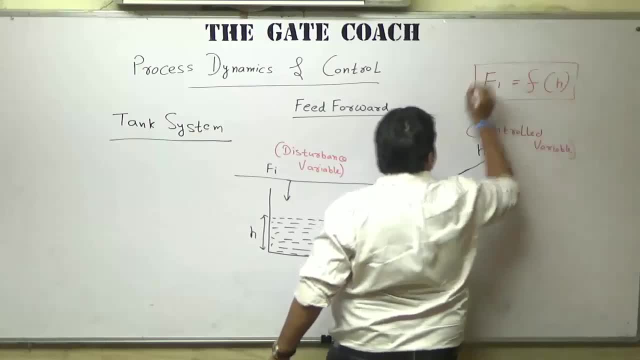 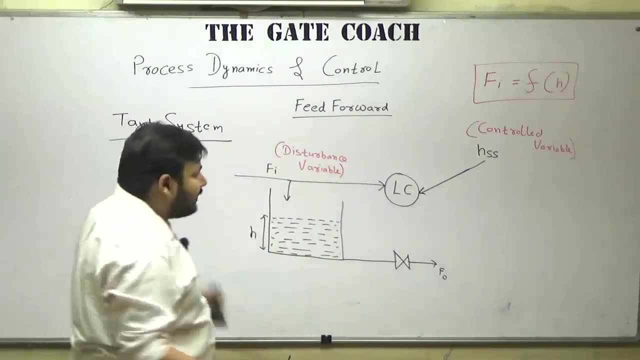 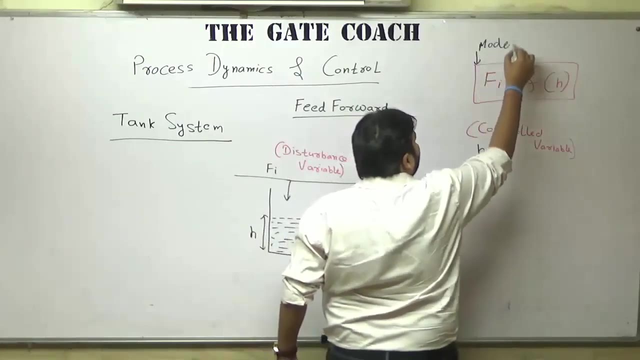 And the height. We need a relation Now to get that relation. How to get that relation, How to generate it Again, that is. That is a different topic. If you want, I will make a separate video on that. So that is a model that we need. 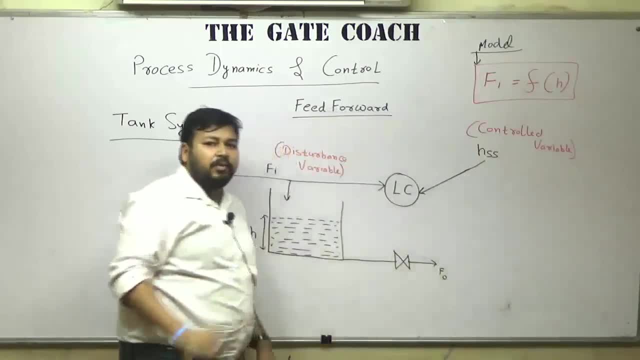 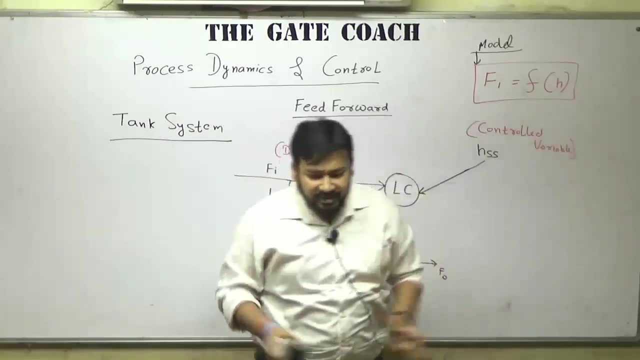 So I am assuming here for the time being That I have the model. That means If I have H, I can get F I. If I have F I I can get H. I have the relation Between the two variables. 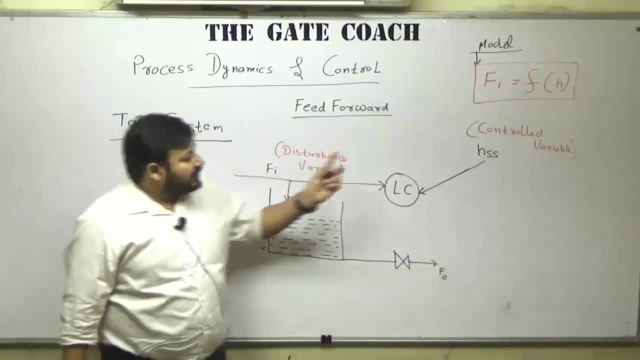 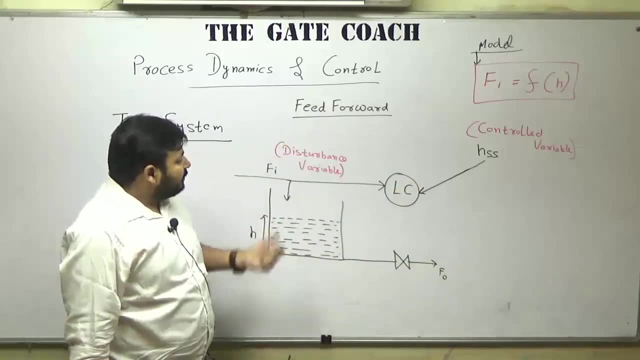 Another point is Where to put this model: To convert HSS into F? I Or to convert F I into HSS. So model can be put anywhere, But the thing that we need to look is This: F? I Is not a constant value. 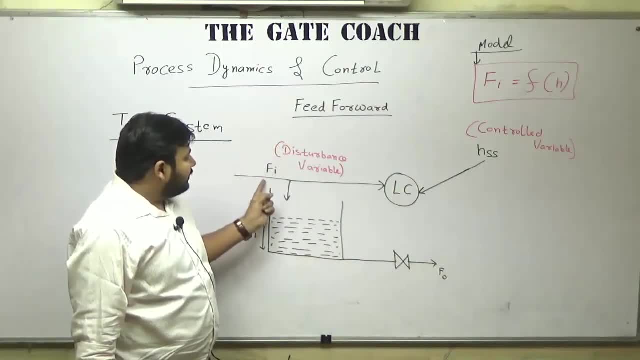 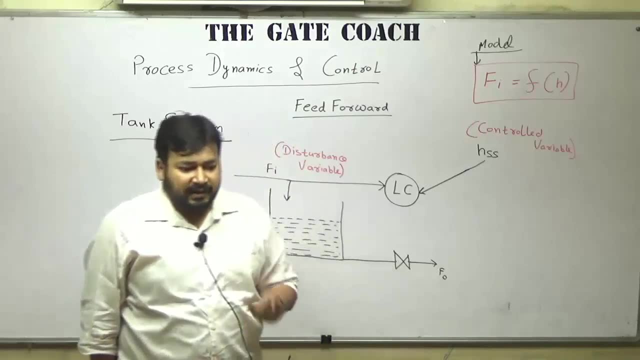 And you can say This: F? I Is not in our hands. That is disturbance. And disturbance means The variable That can change Independently. That can change, You can say automatically So from where This disturbance is coming. 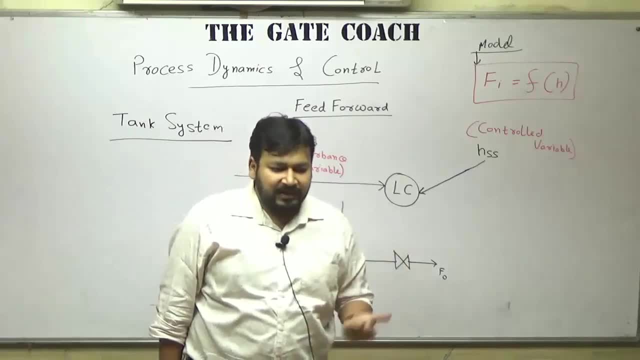 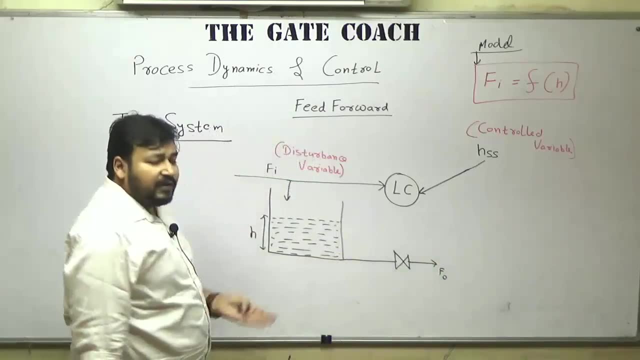 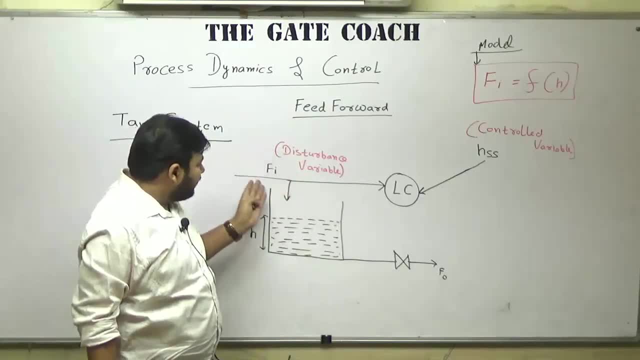 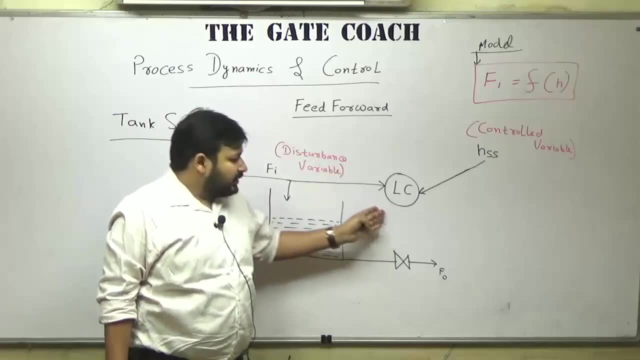 We have No Power to change it. This will change On its own. So if its Change on its Own, The value that will Enter the controller Will change again. That means, If I put a model here, 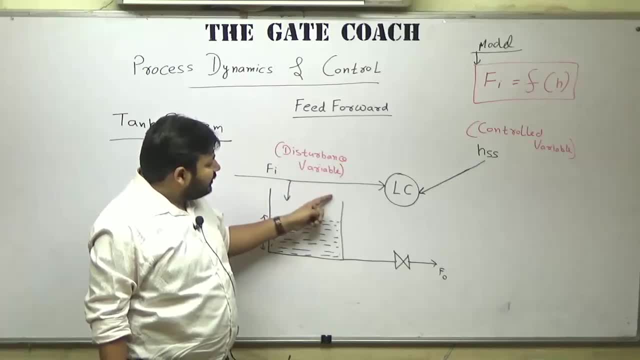 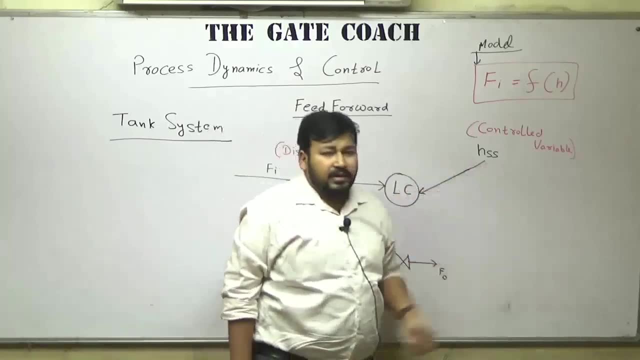 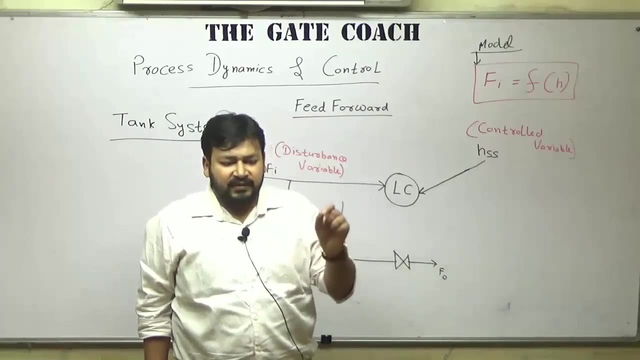 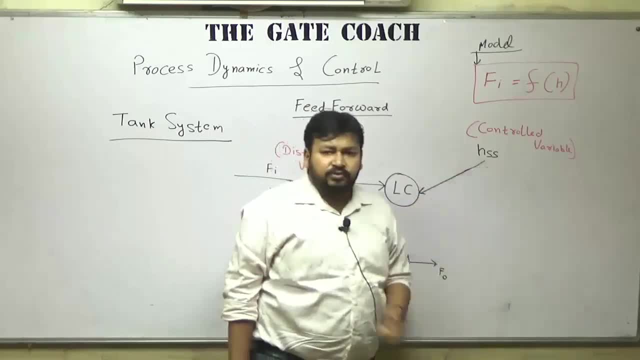 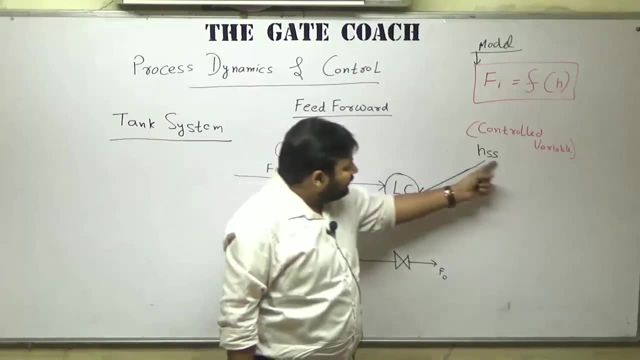 will remain the same. that means if I put it to be equals to 6 meter, it will remain 6 meter. if I put it equals to 6 feet, it will remain 6 feet. so it depends upon me. that means whatever is the value corresponding to this value, there will. 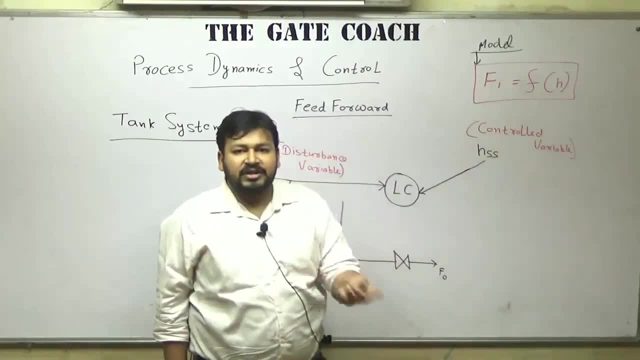 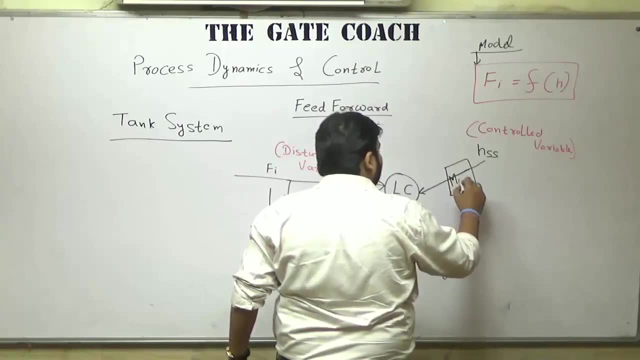 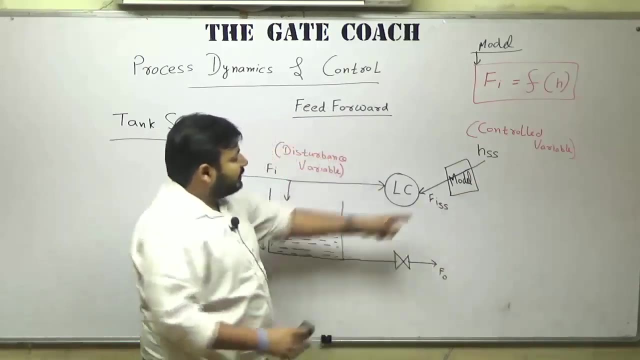 be a fixed value of fi that will not change again and again. so if I put this model here, if I put this model here, then it will give me a desired that will remain the same. so there is no need for the model to work again and again. so in. 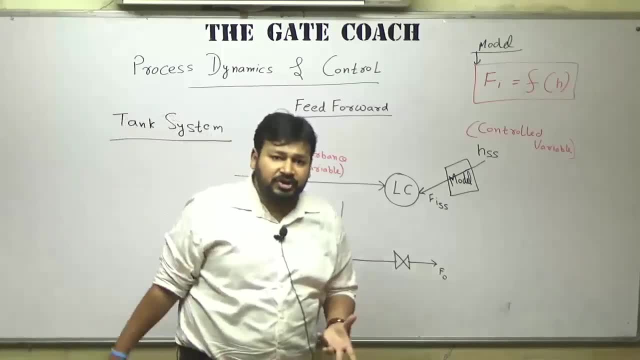 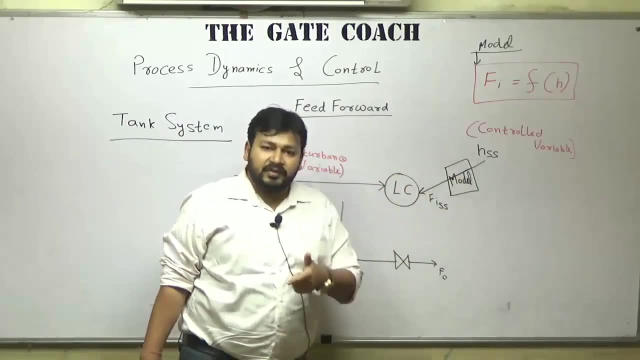 the case of feed forward? that's again a very important interview question: what we do? we change disturbance to set point or we change set point according to the disturbance. so the answer is: we change set point variable to the set point variable and we change the set point variable to the set point. 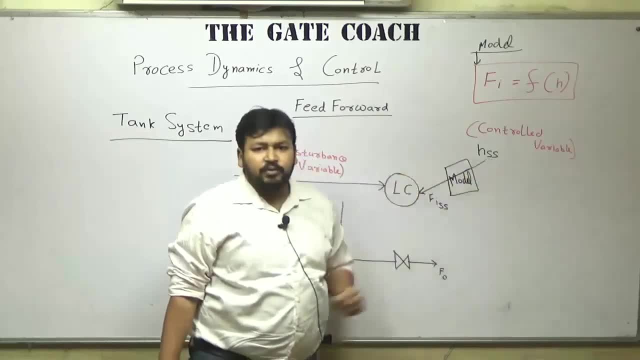 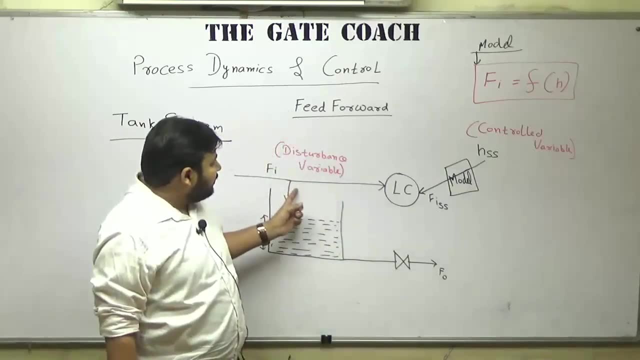 according to the disturbance variable, because set point variable is a user input value that will remain the same and there is no need to convert it again and again. well, in the case of disturbance variable, we need to convert this disturbance variable according to the set point variable again and again. so 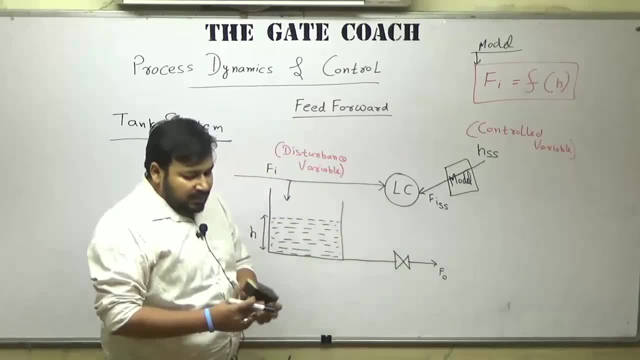 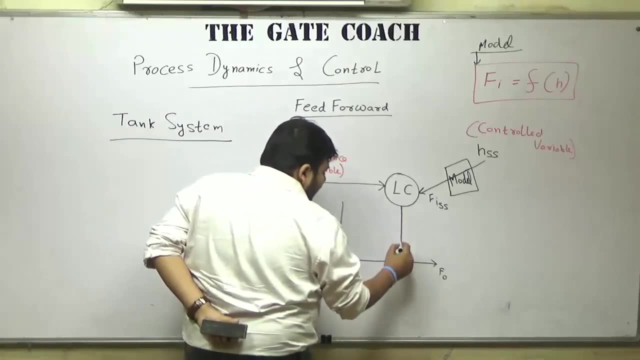 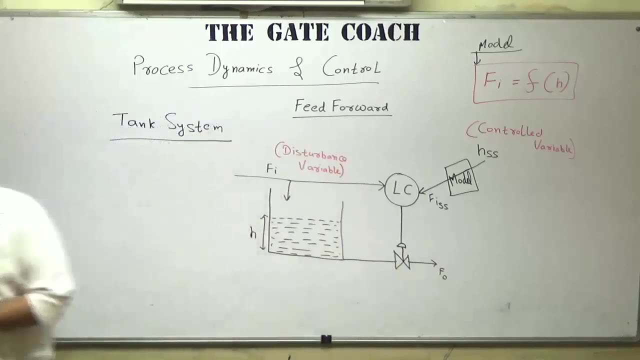 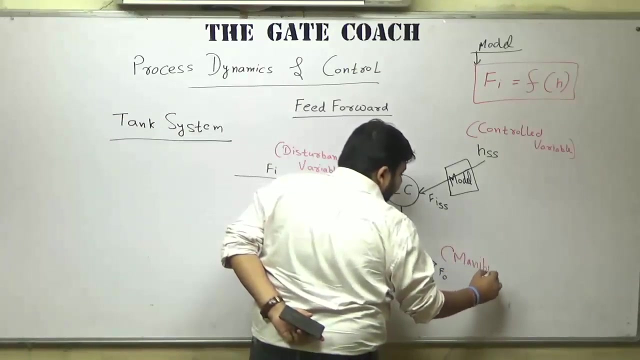 after this: now we can easily take the difference between the two, and by taking the difference there will be an error, either positive or negative, and that error now works perfectly, works on the wall. that will change the value of f node. so f node remains our manipulated variable. so this will remain our manipulated variable. so now you may. 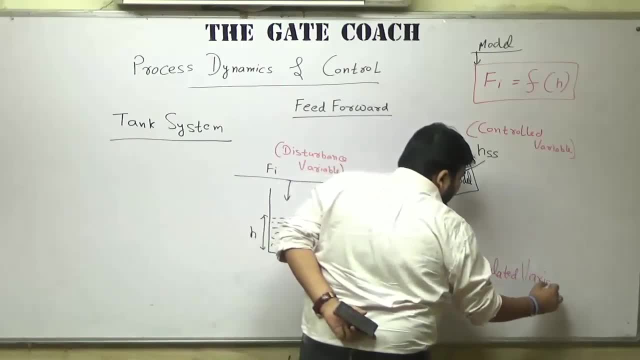 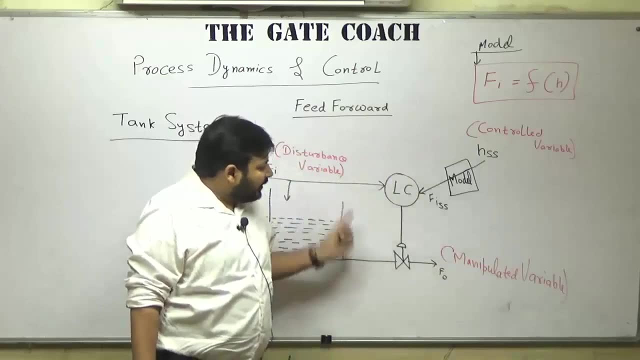 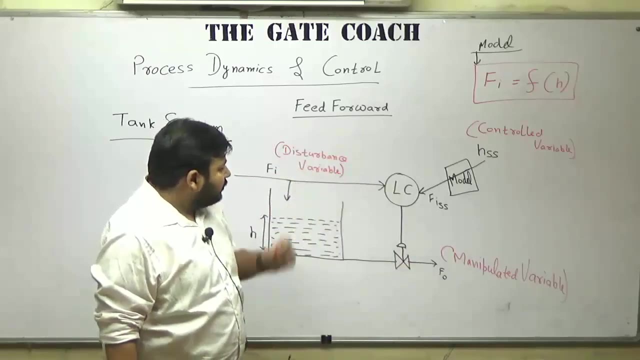 wonder that, if you compare the feed backward with the feed forward diagram that I drawn, in the feed backward there is control, there is measured, there is manipulated. but here there is control, there is disturbance and there is manipulated where is measured. So the variable that we measure becomes a measured variable. So here, in this case, 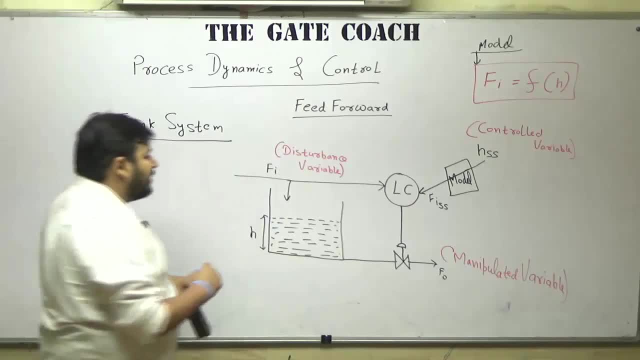 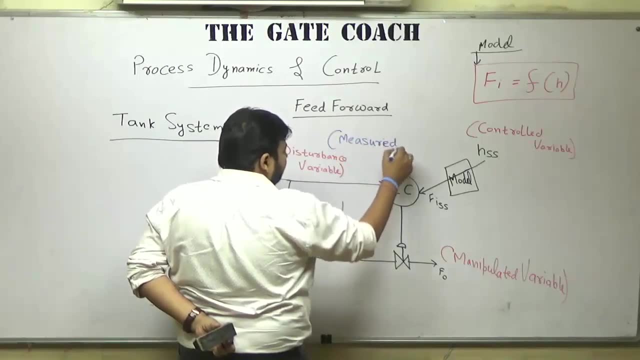 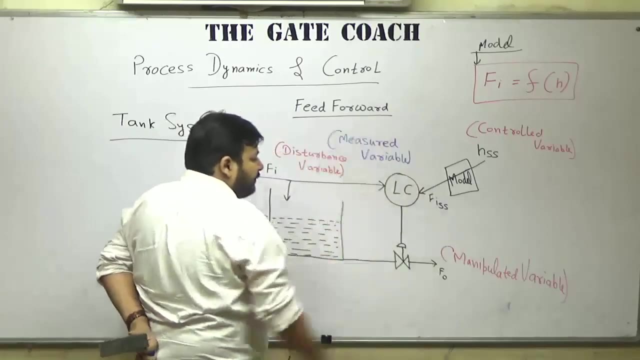 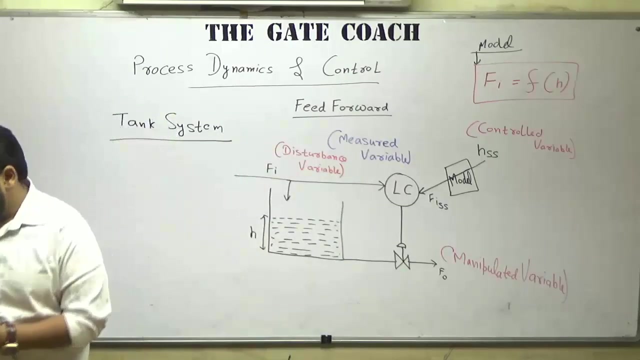 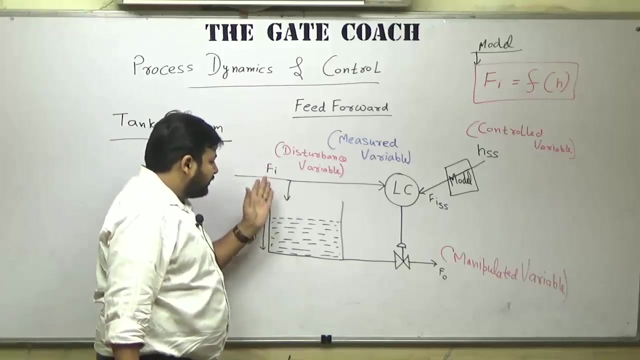 our disturbance variable is also our measured variable, because in this case we are measuring the disturbance, So controlled, measured and manipulated, and this type of strategy now is known as feed forward control strategy. So in the feed forward, what is there? that if there is any change in the feed flow rate, or in the surrounding or in the input, or if there is 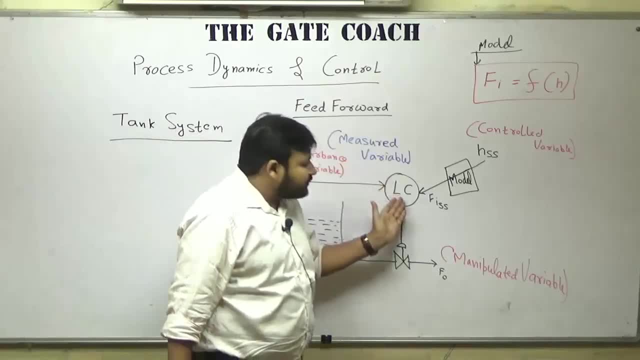 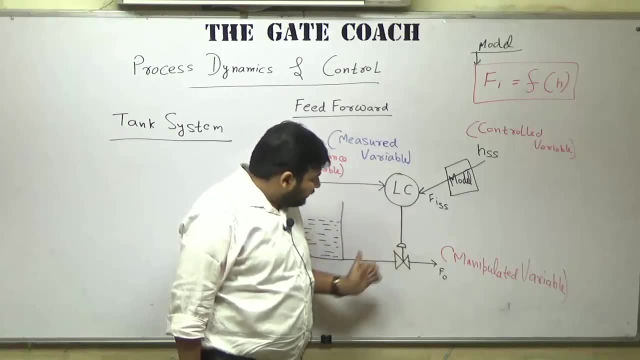 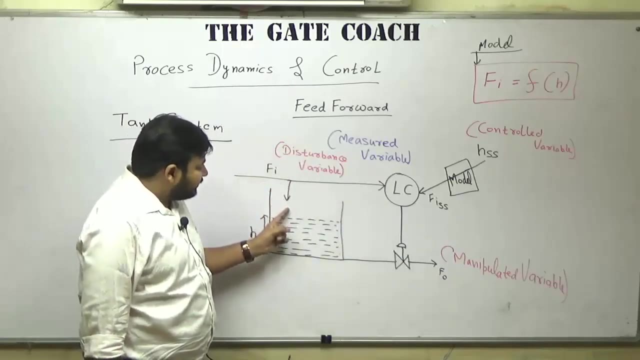 any disturbance, then that disturbance is sensed by the controller, and controller will give its best to prepare the system according to this change, by the help of valve, so that when this disturbance ends So the system is ready to balance the changes, to counter the changes, such that the ultimate 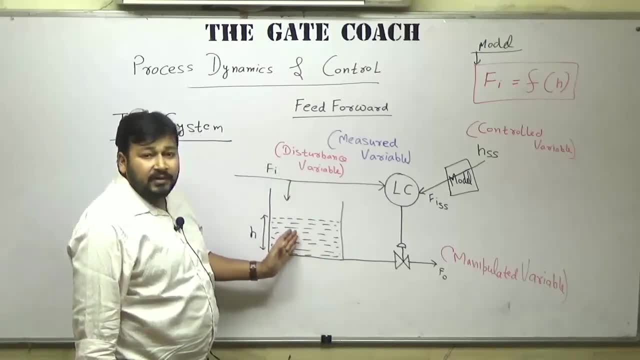 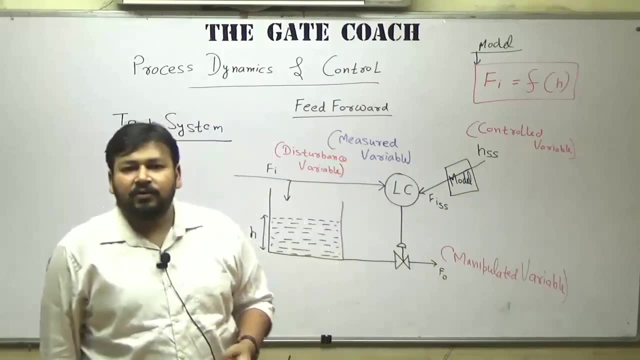 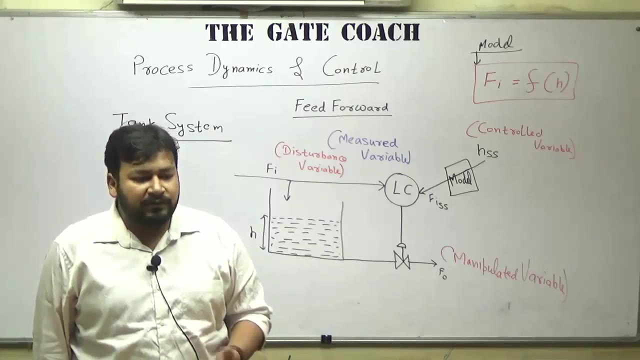 height after the entering of the feed will remain same, that is, equals to HSS. So this is known as feed forward control strategy. So if I talk about in life, what is the way to live life, the way to live life should be feed forward. That means, whatever the challenges, whatever the problems. 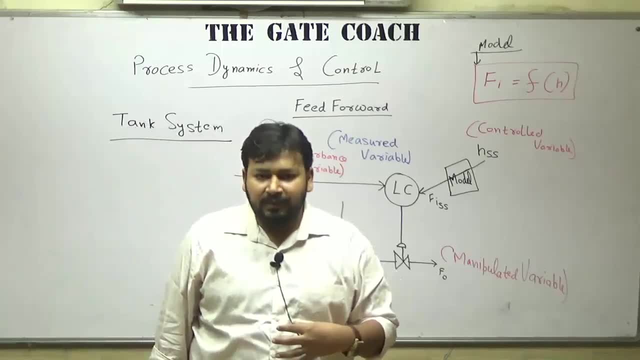 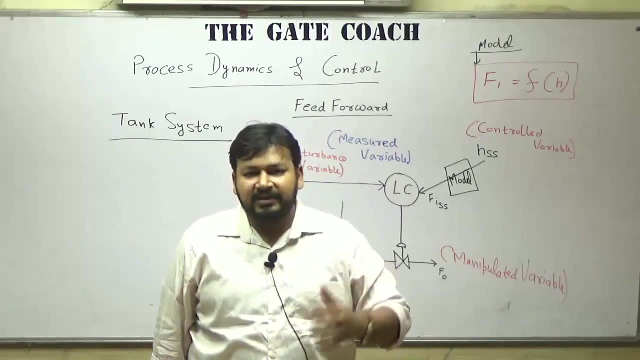 they are going to face. they are going to face the same way. So if I talk about in life, what is the will gonna come in our life. we know it because if we don't do the work that is required to be done presently, then ultimately the challenge and the problem will gonna come. so some problem can be. 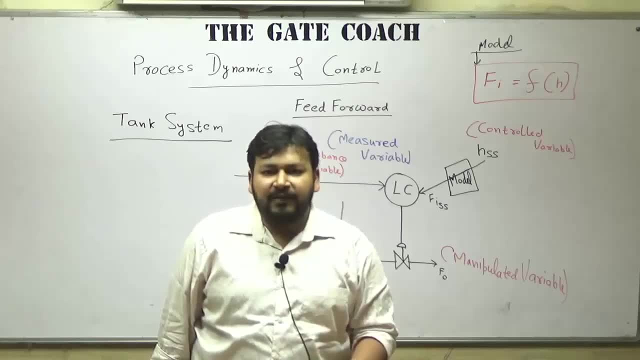 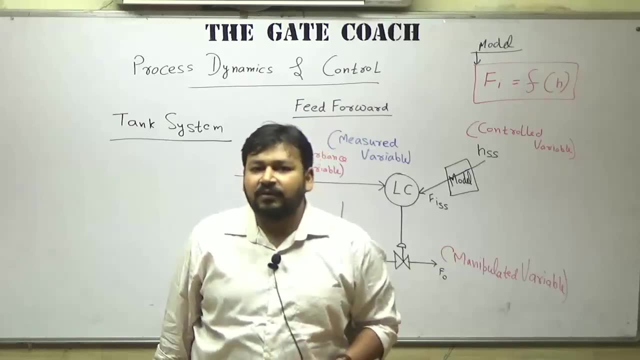 identified. some are not, but those that can be identified we can prepare ourselves for that. we can prepare ourselves for those challenges, and if we do that then the steady state of our system will remain the same. but if we go according to the feed backward, it will cause some things, that is. 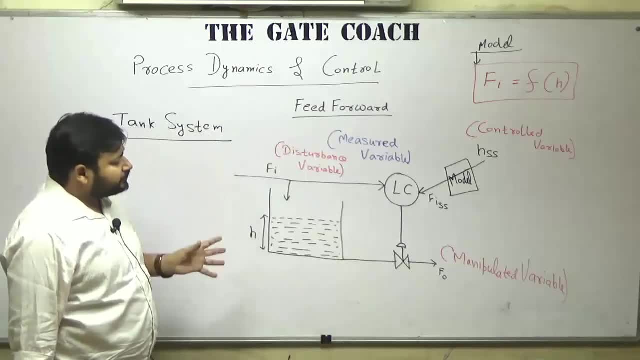 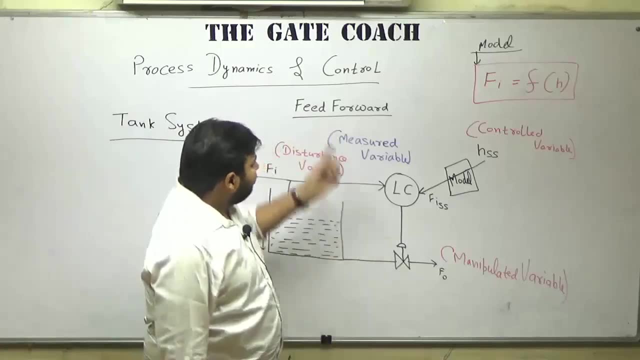 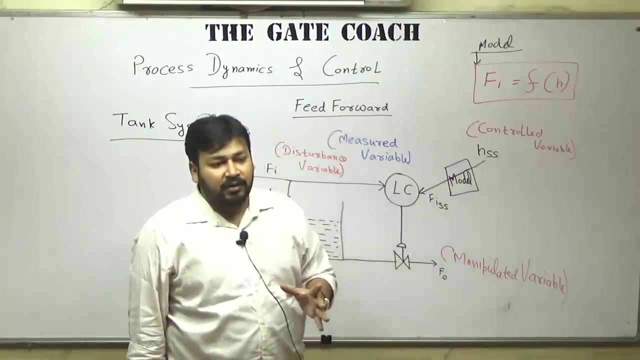 not desired. but in the case of control system, what strategy we should follow? ideally, we should follow feed forward, but in the diagram you can see that if we follow feed forward, what i need is the model. this model is necessary. without this model, we cannot apply the feed forward control strategy. 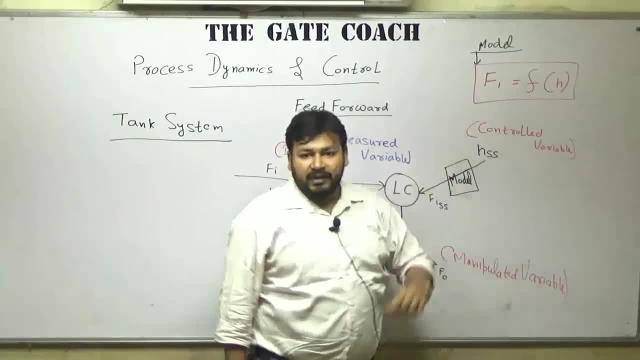 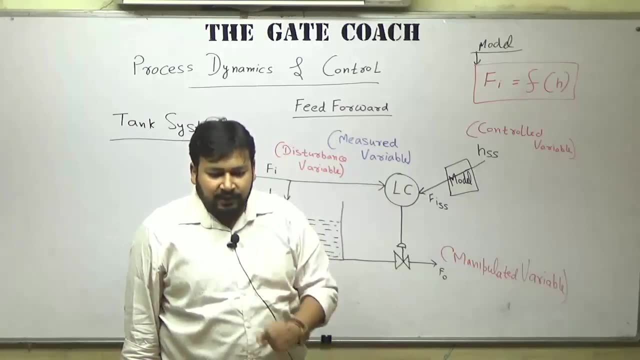 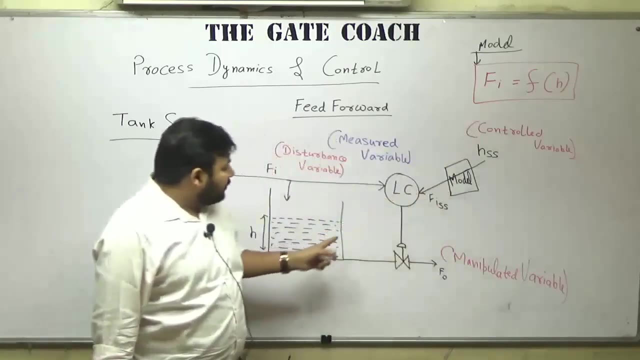 and if this model is not available, feed forward strategy cannot be used. and if this model is available but the accuracy is not 100, then again there is a problem, because if accuracy is not 100, the system will be ready, but not exactly, to minimize the error. that means 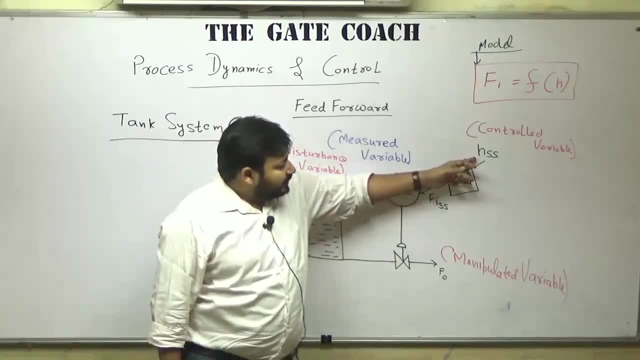 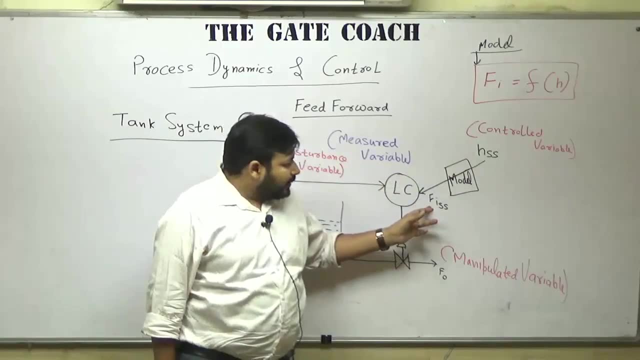 if let's say the height is 5 meter and according to that 5 meter height, the conversion should be, let's say, 3 meter cube per second. but because the model is not accurate, this value is not 3. this value may be is 2.8. so this 2.8 minus this value will generate an error. but in the real case this: 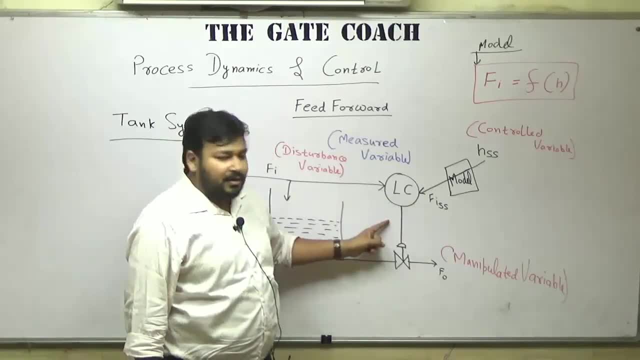 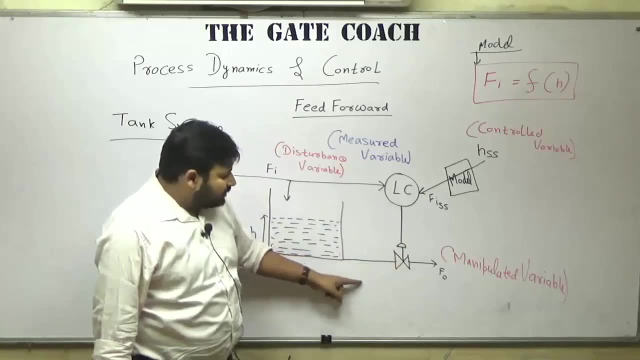 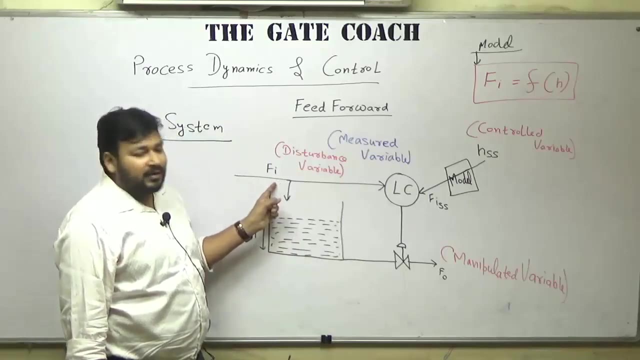 3 minus. this must generate the actual error. but now the error that has been generated is wrong and this wrong error will do the wrong action and this wrong action will prepare the system wrongly to counterbalance the feed flow rate. so what will happen? the overall height will not. 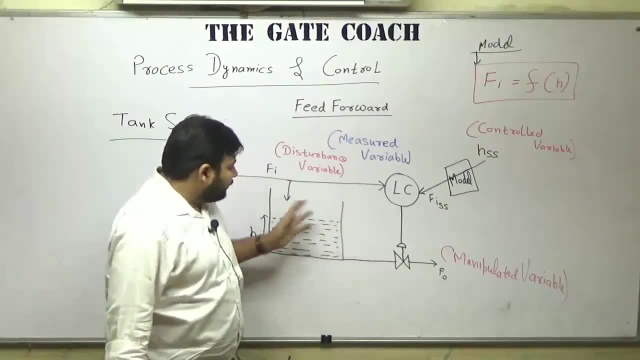 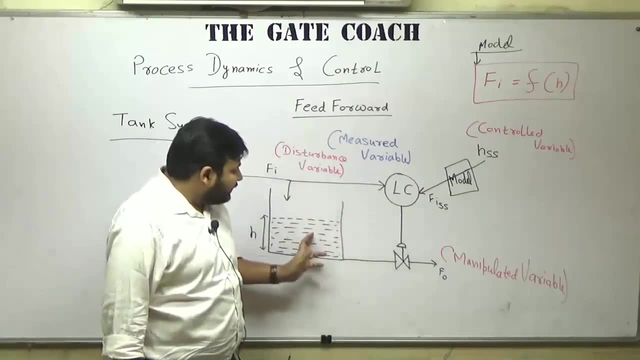 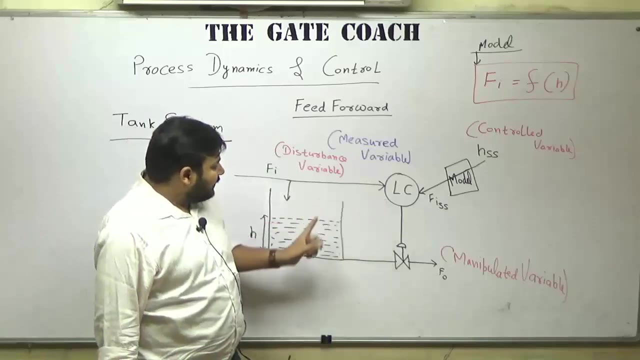 be equal to hss. so what will happen? this overall height will not be equals to this hss and there is a permanent instability will get entered into the system because this controller does not know what is happening inside the system. the controller does not have any knowledge. what is there in the system? 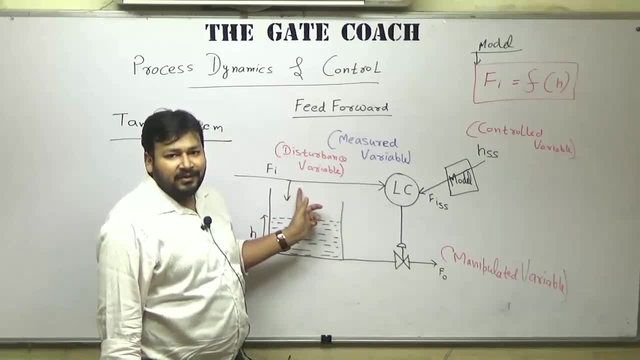 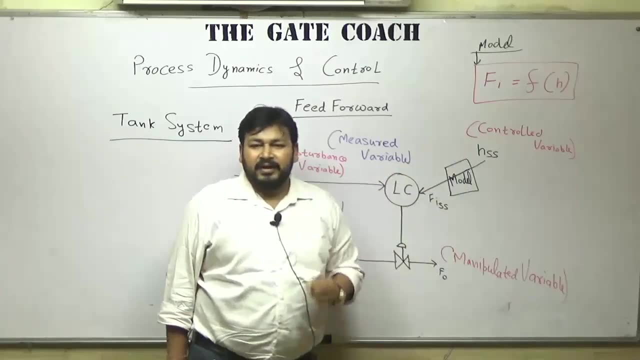 it just dealing with the changes in the disturbance. so if there is any wrong action taken then that height will never be equal to the hss. so that is the most, biggest, biggest disadvantage of the feed forward control strategy: that it generates the permanent instability in the system. if the 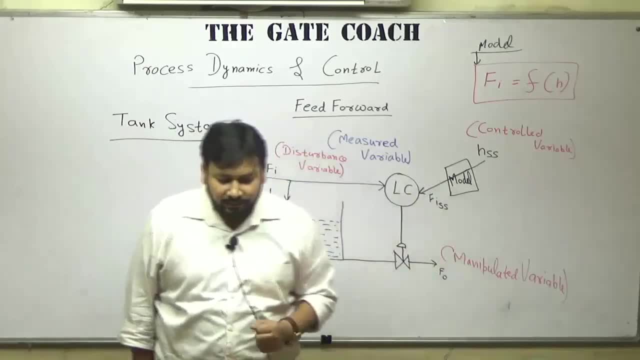 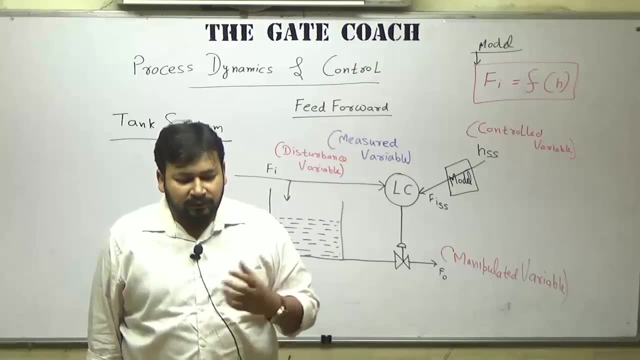 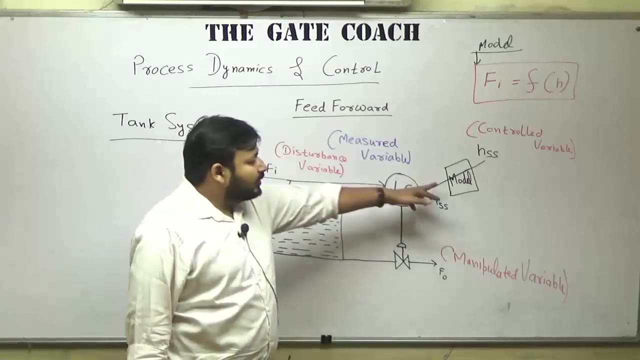 model is not 100 accurate. so that is why in our chemical engineering processes or practices, 99 of the time we use feed backward control strategy. because in the case of feed backward control strategy there is no need to have this model, there is no need to have the knowledge of the disturbance.